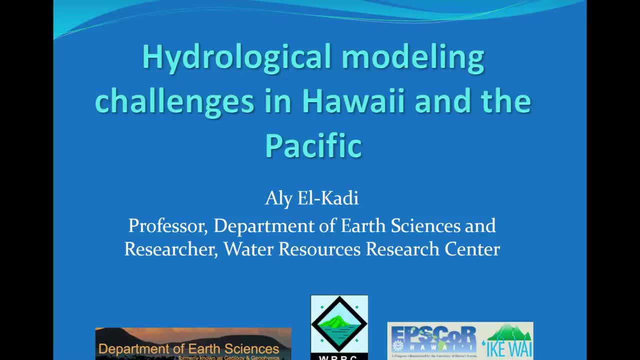 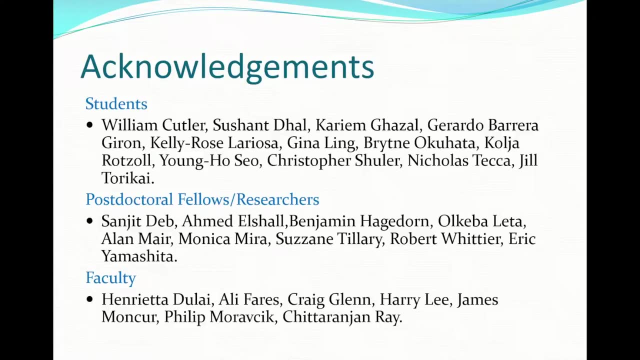 It's about hydrological modeling challenges in Hawaii and the Pacific. I'd like first to acknowledge the support I had over the years from students, graduate and undergraduates, as well as researchers and my fellow faculty members, Especially students. They have done a great job over the years. 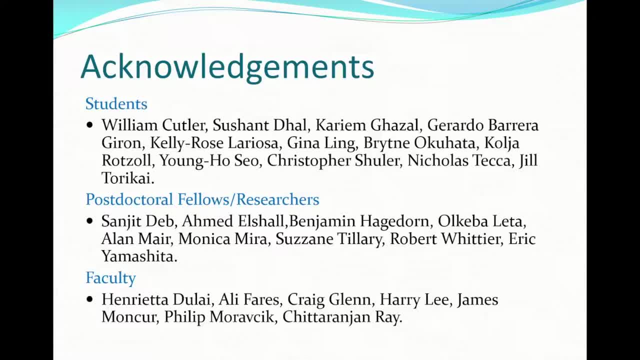 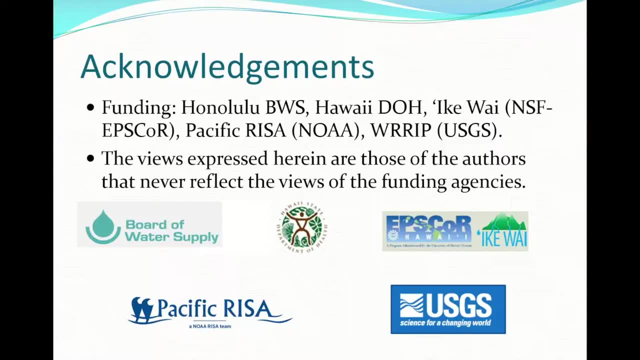 I'd like to especially to acknowledge the high productivity of a number of them, including Bob Whittier, Collier Russell and Chris Schoeller. I'd like also to acknowledge the support of the funding agencies. here in alphabetical order: the Board of Water Supply, the Hawaii Department of Health, EBSCOR- through EQI Pacific RISA and the USGS. 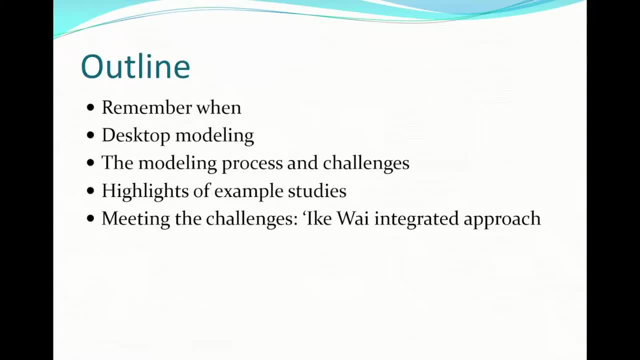 Okay, here is the outline of my talk. We'll talk a little bit about history, then talk about advances in desktop modeling, then talk about the modeling process and the challenges associated with it, then highlights of some sample of my studies and end up with update of EQI research. 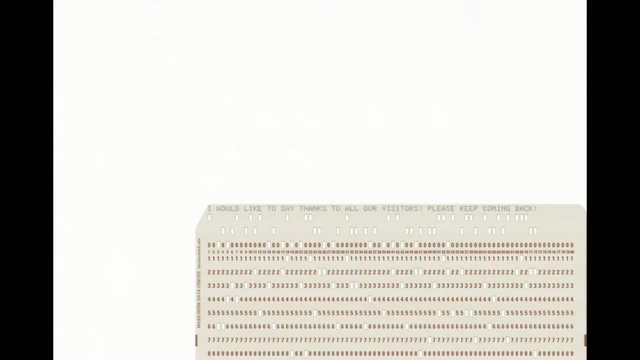 Okay, so I go back to a little bit of history. I'm sure some of you remember this one. Okay, so I go back to a little bit of history. I'm sure some of you remember this one For the younger generation. this is called punching cards. 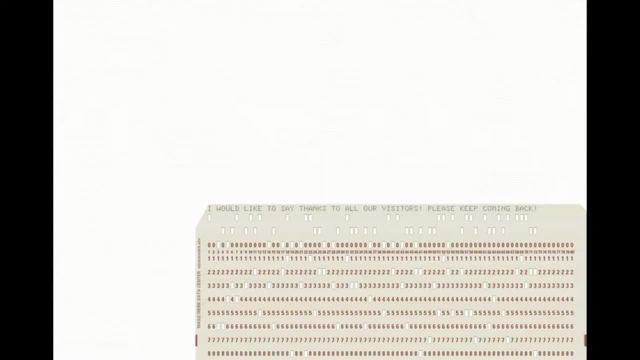 And we used to use this for writing software. So, for example, if I have a short program like this- assemble and calculate the area of a circle, So here I will read the radius of the circle And here I calculate the area, then print the results. 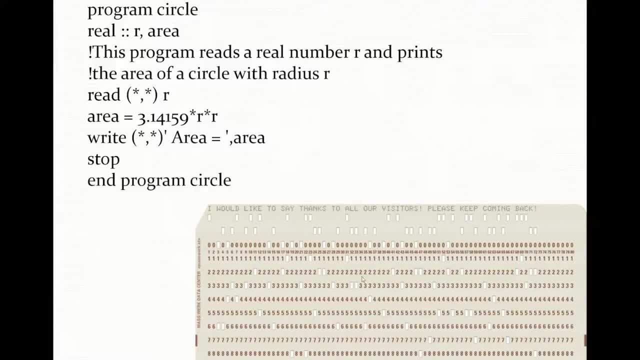 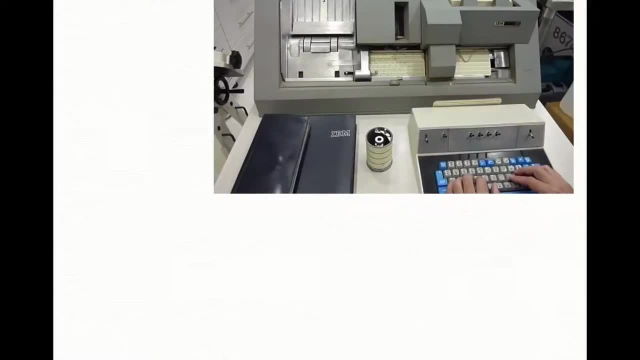 So this is nine lines program, So I will require nine cards like this. Then here is the machine that we used to punch in the cards, And this is like a typewriter kind. Then here is the cards, and you do it one by one. 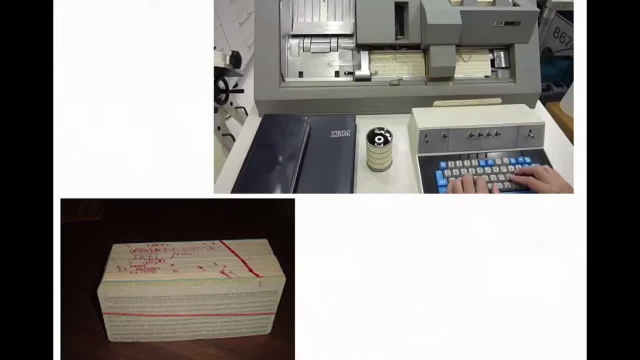 And basically I used to go at night so that I can find room to type in my cards. This would be a typical deck of cards for one specific software And I assume this marker line here is intended in case you drop the deck, So you can at least get some idea about the order to sort them back in the correct order. 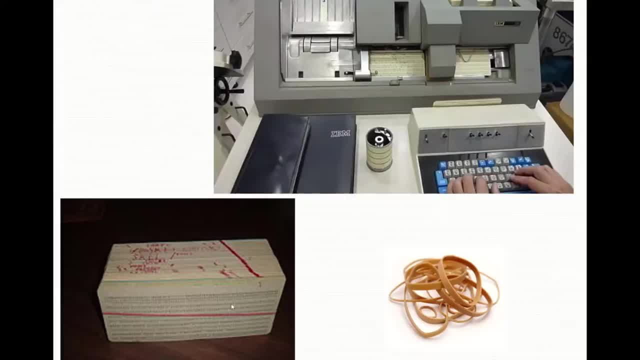 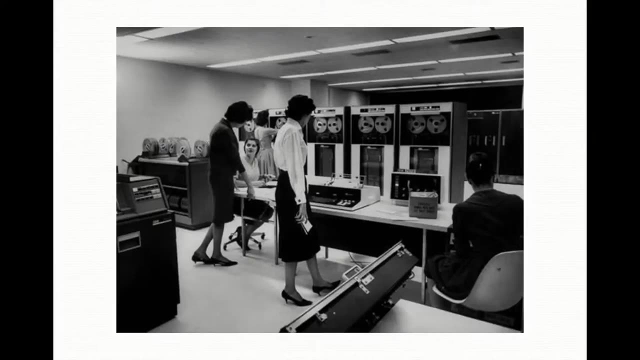 And you should have plenty of these and make the L strong enough to keep this deck in order. Okay, so here is you, handed over to the formally dressed person. So the first program, or computer operators. then they feed it to the card readers. 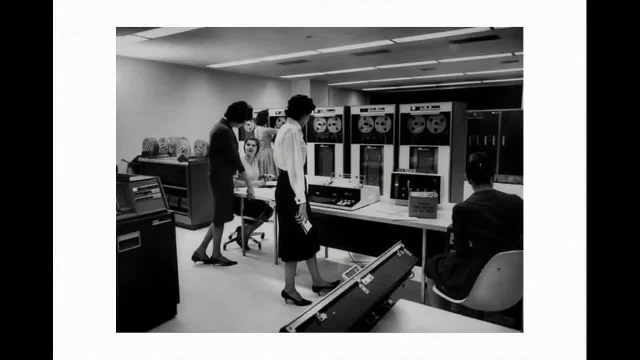 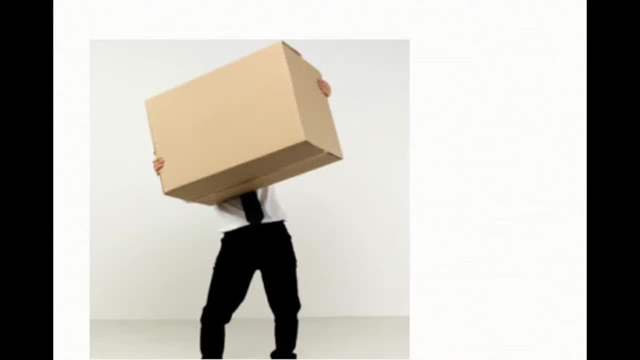 Then you hope they are not stuck or something wrong that we will have to feed it again. Then in the next day you found your results wrapped on your hard copy. And now, in case you are moving after your studies, this is, I assume, after four years of graduate studies, including classes and research. 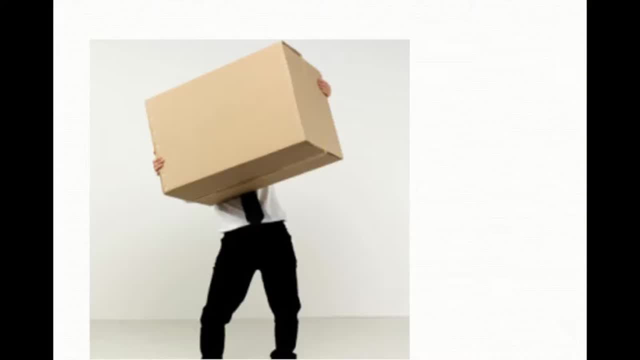 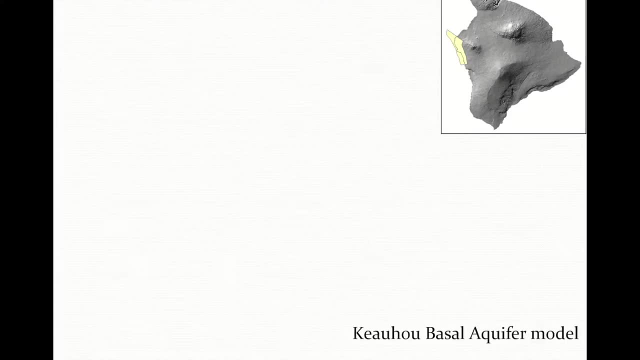 This is how you will be carrying your software, And I assume one of these could have done it for us. Okay, now go to present. Just first forward to what we have now. So this is like a site on the big island. It's called Kehoe Basel Aquifer Model. 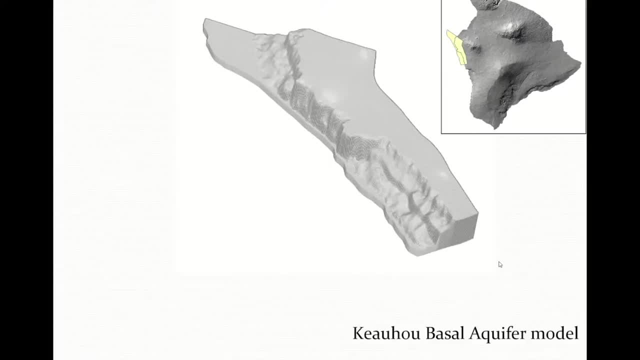 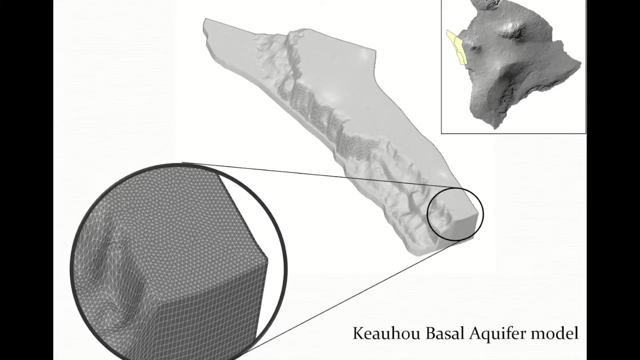 Here in the side of the island, I can use very quickly in my desktop the software to create a three dimension View of the site- Then if I'm using this numerical analysis, like, say, using the finite element method. So this would be a number of elements. 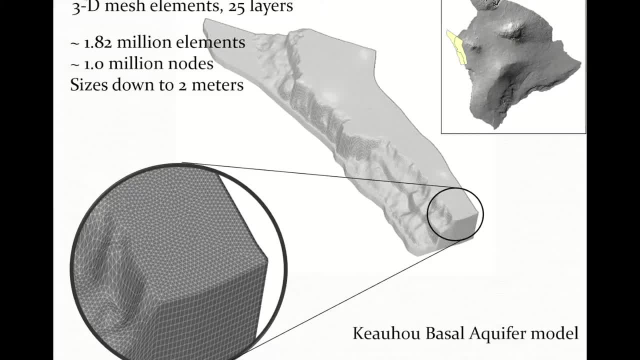 And I can go for very high resolution, like for three dimensional mesh: 25 layers. I needed, or I can design for more than 1.8 million elements- This little things here- And 1 million nodes, which are the points at the corner of the triangles. 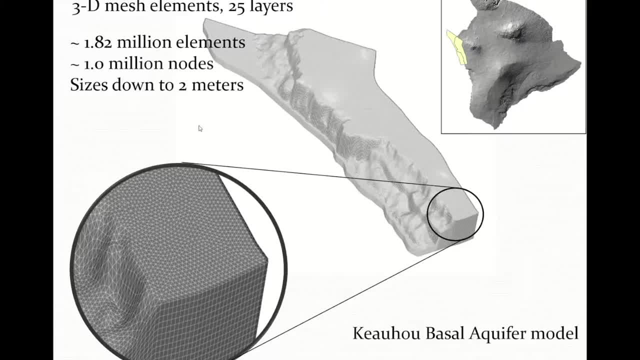 And I can go to size it down to two meters And if you're familiar with numerical method, this is how number of equations that you need. So I need to solve 1 million simultaneously simultaneous equations And they can be nonlinear If you're dealing, for example, with density dependent flow. 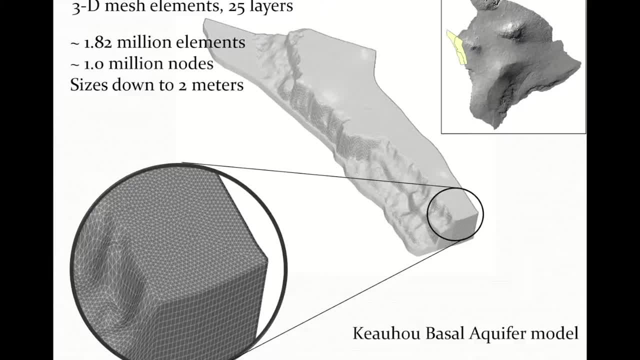 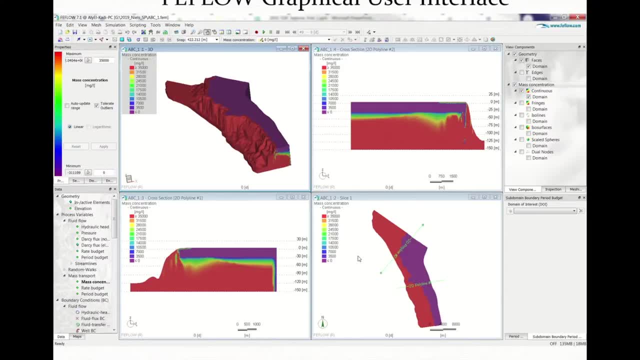 They can, you know, take time, But they're still possible to do in your desktop Something we could have never done years ago. And this is a screen how it looks like for some software. It's called the FIFLU And this is your results screen. 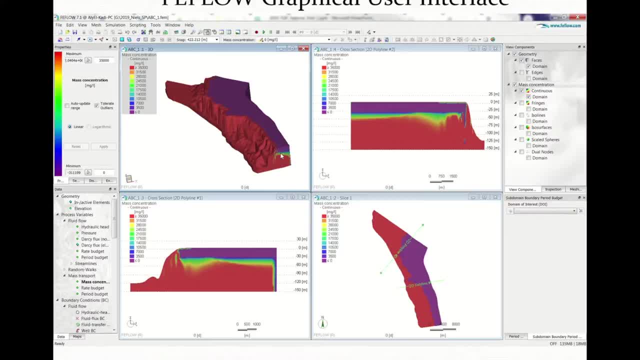 So I have a three dimensional view. They choose the extent of the salt water length Or the salt water distribution in the aquifer, And this is the cross sections And this is blend view. I can show the salinity profile at different levels. 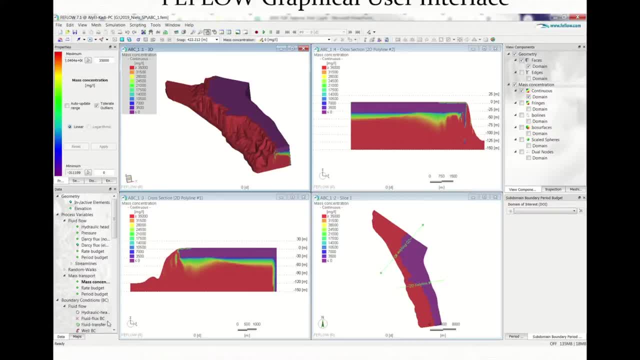 So all the data I have, all the results, can be manipulated from here. I can just basically select what I want to display And I can communicate with maps. So if you click over this tab here, You can see all kind of maps that you can import to the system. 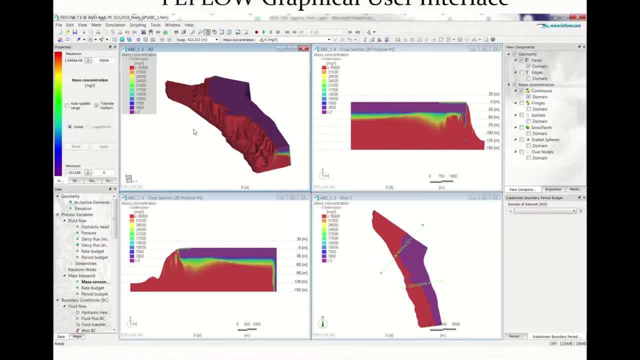 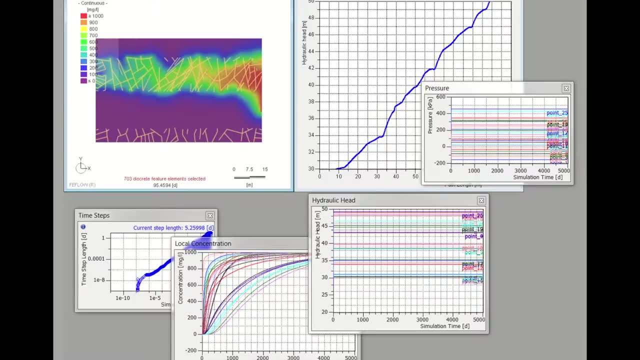 Like GIS maps, where you can read the data And to integrate it Relatively easily in your model. Then here is what is good about it Is that you can monitor everything live, Like here. I can look at the salinity, I can look at the hydraulic head. 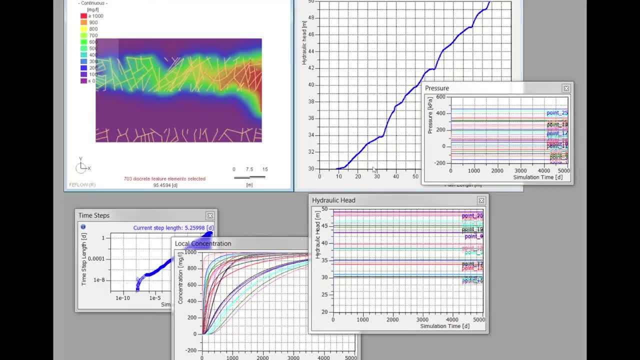 I can look at the pressure. I can make cross sections. This is all while the program is running, I don't need to stop it. I can also look at the size of the current- You know- time step for simulation. I can adjust if I have trouble or problem. 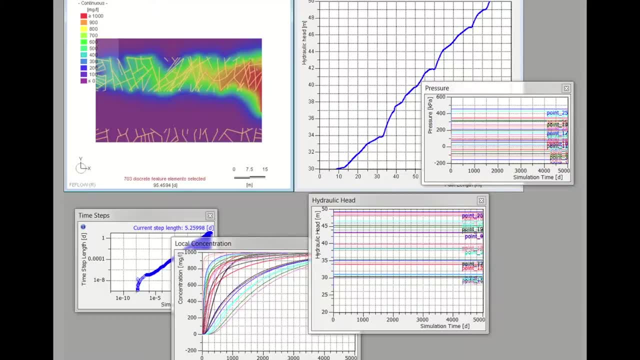 I don't need to stop the program. sometimes I can pause it Or just make changes, Or I can save the results at certain times And I can recall it anytime. So if it crashes, I can go back and restart. So you don't have to lose what you are doing. 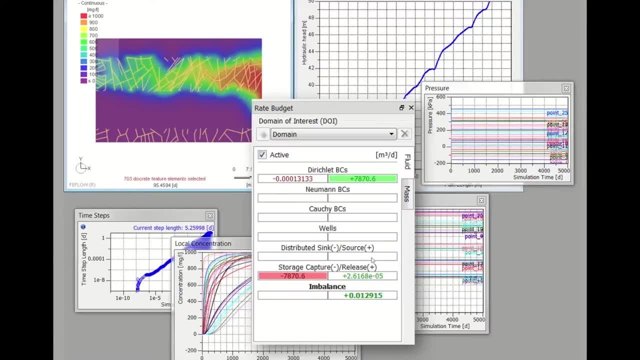 A nice also feature. I can look at the water budget Dynamically All the time And see if the model is behaving correctly. If not, I can stop it obviously, So I don't have to wait hours and days And restart. 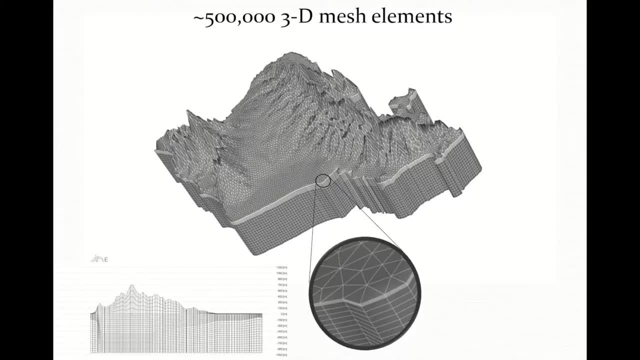 This is an example of a model for the whole island of Oahu. This is relatively coarse, About 500,000 mesh elements, And this is how they look like. This is like 40 vertical layers And this is a close up to the finite elements. 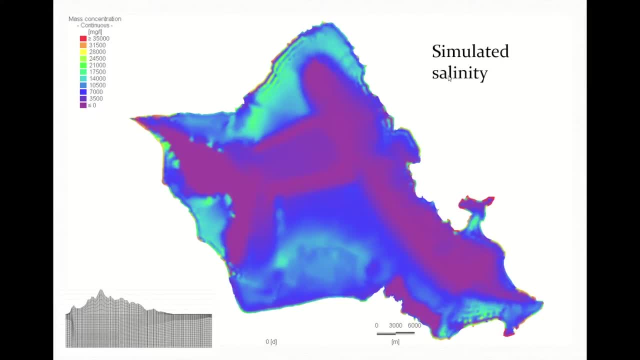 And here is quickly the results. I can look at simulated salinity at different depths, So this is basically close to the surface. So we have fresh, Which is here is a purple color, And the blue is fresh. And as I go deeper, 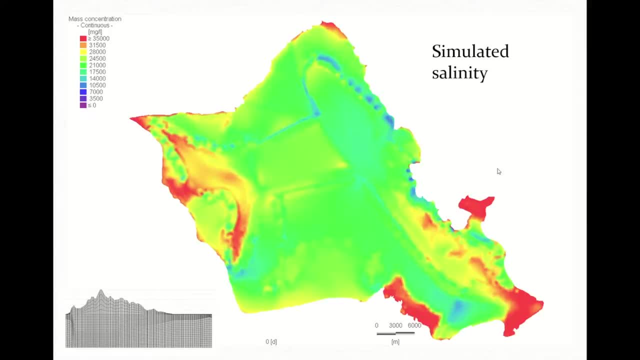 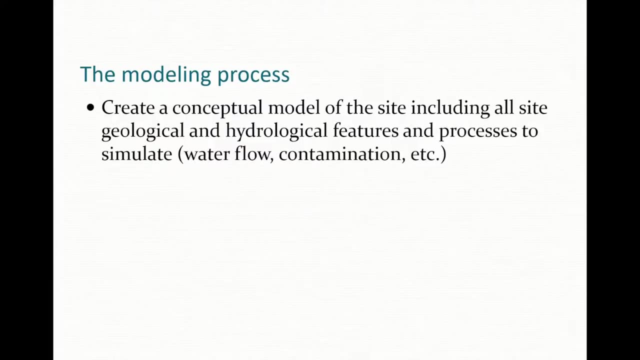 So you can get into higher salinity And higher and higher, Until you get to the salt And you get to the water. So exactly what is the modeling process? The first step is to create a conceptual model Of the site That includes all the site information. 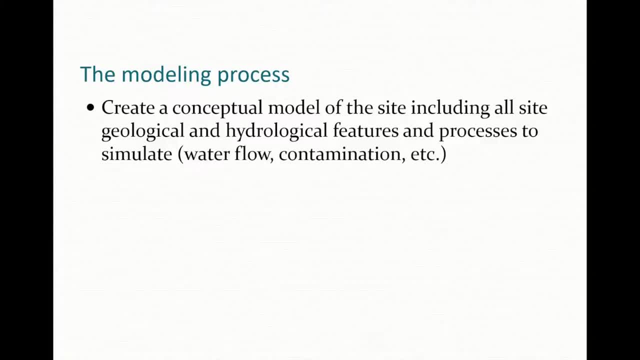 Geological and hydrological features And decide what processes you would like to simulate. Usually we would simulate water flow And contamination. Then, after that, you create an American model And we will simulate the processes Which are the water flow and contamination here. 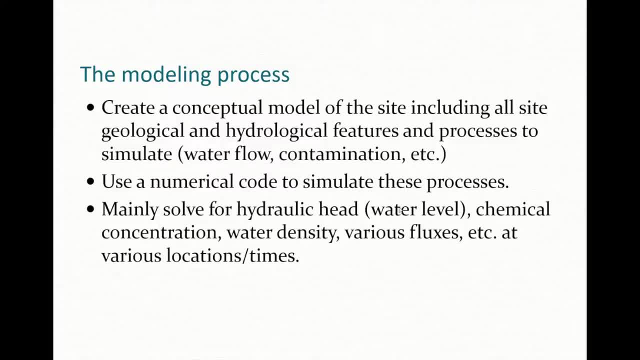 Then I can solve for that, For the hydrologic head of the water level Or chemical concentration, And I can simulate also density, Various fluxes At various locations and times. Then, after you create the model, You do some validation Or calibration validation. 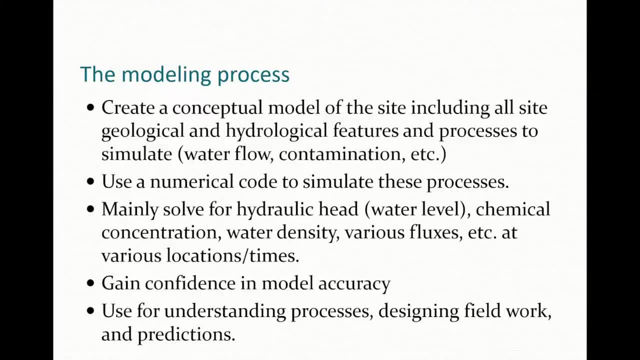 You gain confidence in the model And apply the model. We can apply it for understanding processes, Designing, field work And predictions. That's something good about models: You don't have to wait for a site for years. You can study it in your comfortable office. 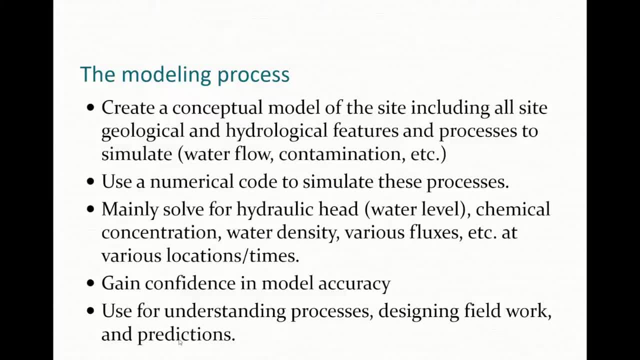 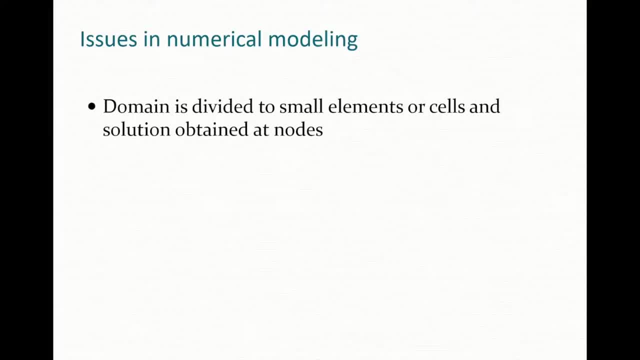 You can do simulations for thousands of years And do some scenarios if needed. So some important issues. As I showed before, The model area is divided to small elements Or cells, And the solution updates at the nodes. The solution requires solving a large number of equations. 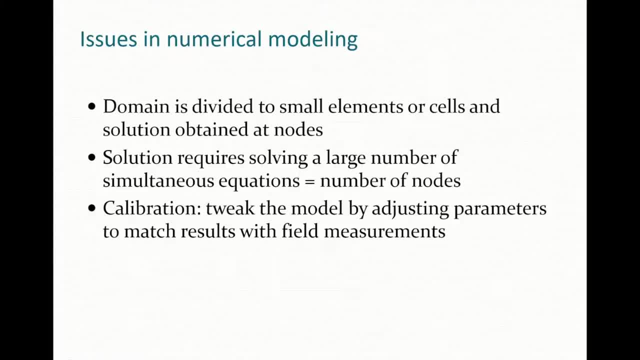 As I mentioned before, And I need something important here, It's calibration- Just to estimate aquifer parameters That can give me the results at known Points or locations. So you change the parameters by iterative process To find out the parameters. 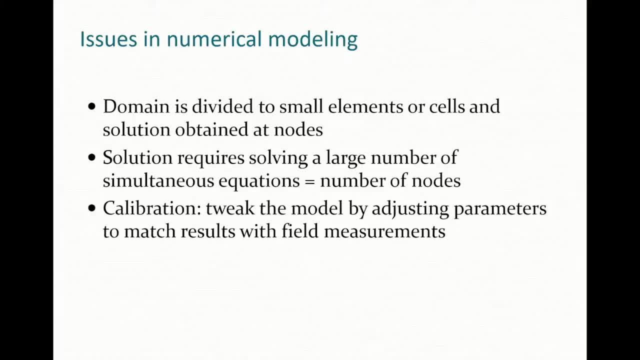 That will match field data with your results And validation is similar to calibration, But you don't have to change the parameters. So once you get the parameters from calibration, You just apply it here And see how accurate the model is. Okay. 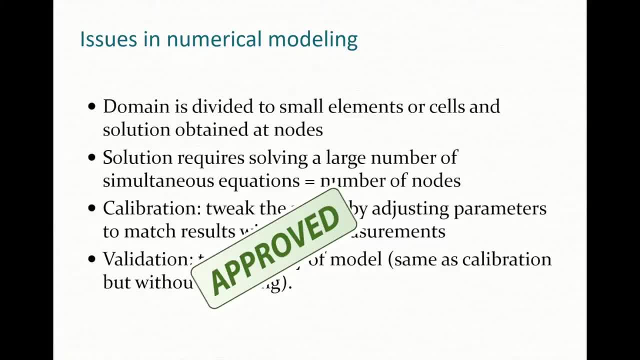 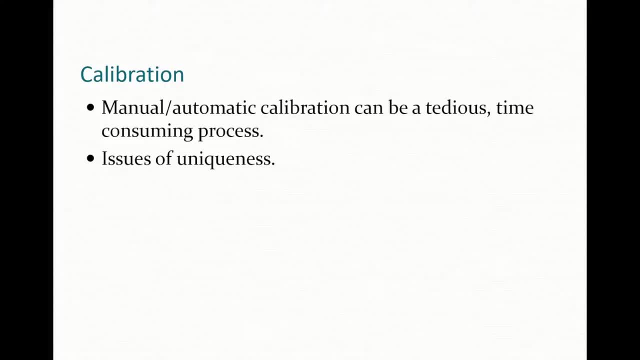 And once you Calibrate And relate, The model is ready for use. Calibration is a very tedious process. It can be done manually Or through automatic process. So manual means you do guesses At the beginning And update or change. 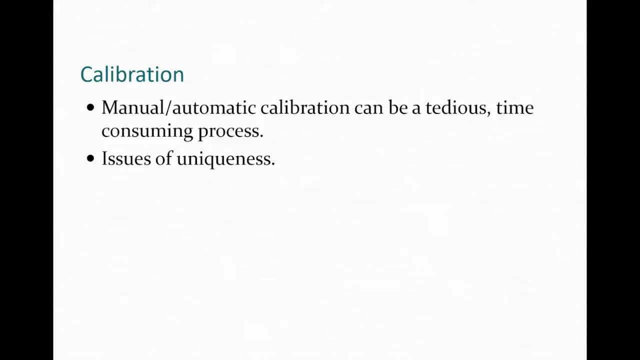 Until you get the match, The computer, more systematically, do it for you Through many iterations And it's basically the same process: Start with guesses And adjust until you get the good match, And it is a very tedious process, As I mentioned. 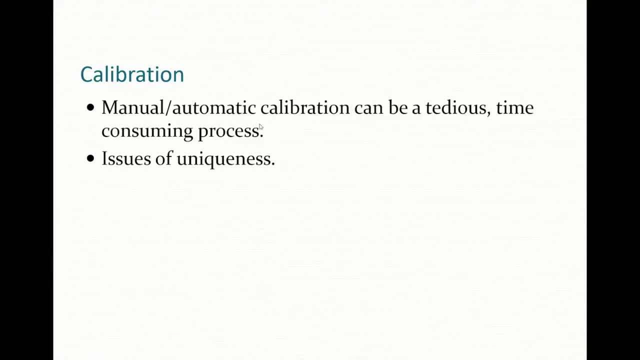 And there is important issues of uniqueness, Like if you calibrate the model for a certain time, Would it be applicable to other times? And also different combination of parameters Can give you the same answer. So aquifer should be unique, But it's not exactly that. 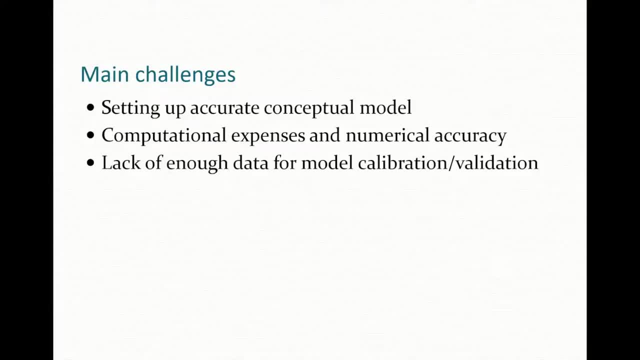 It's a very simple process And it's very easy to do Through model. So the main challenges has to do with creating conceptual model Which is reflects our understanding of what is happening. Then, if the model is high resolution, It will take, you know, large computer time. 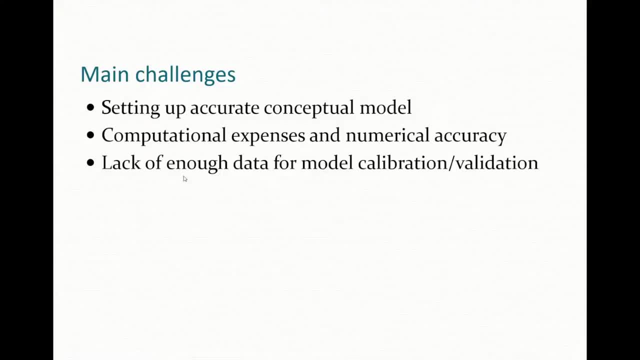 Then, visually, we don't have enough information for model calibration And validation And- this is something important in Hawaii- Issues about data availability And, as I say, Garbage in, Garbage out, Unless you really calibrate the model accurately, Unless you have enough data to do that. 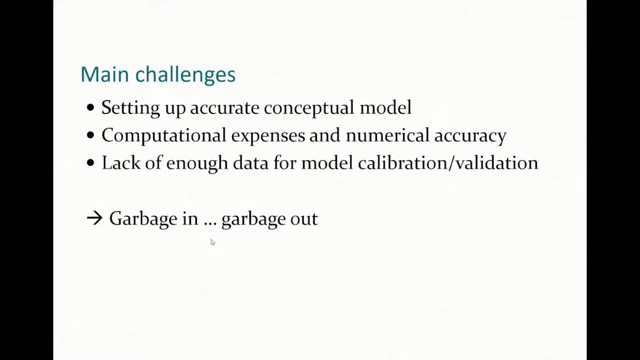 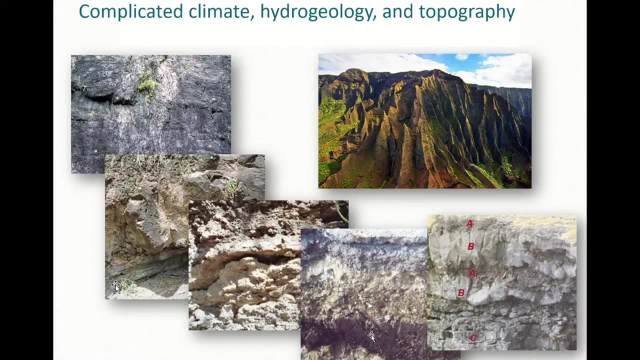 Then it will be. you know, results will be questionable. So here is We have the reasons for challenges in Hawaii. The climate is very complicated. Simply, you know, You need high resolution climate information. Data in one watershed are not applicable. 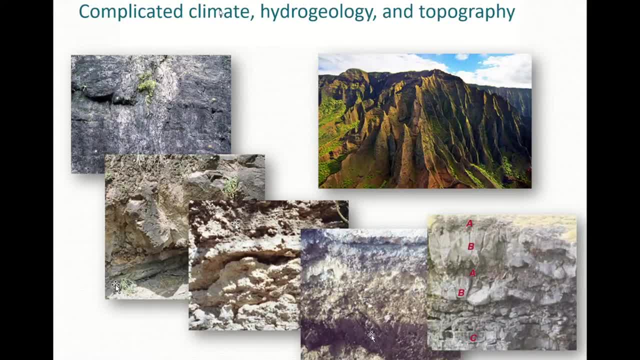 Or can be used for neighboring watershed. The climate or weather is variable, Highly variable, And times and space, So that's affected really in our ability to do predictions. Hydrogeology: As you can see here This is dikes, Sedimentary formation. 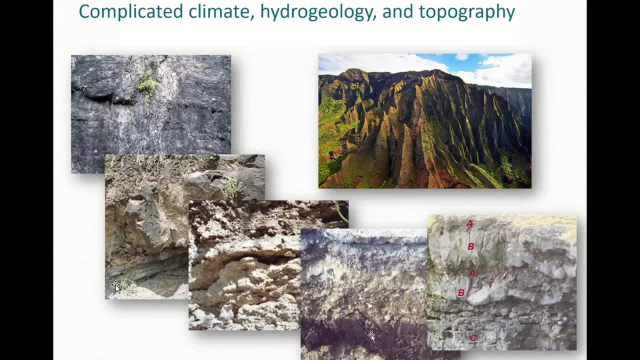 Basalt. They all have high variability And even there is questions about, you know, validity of these porous media models For things like that. Even within basalt, You know there is different layering of different properties, As you can see. 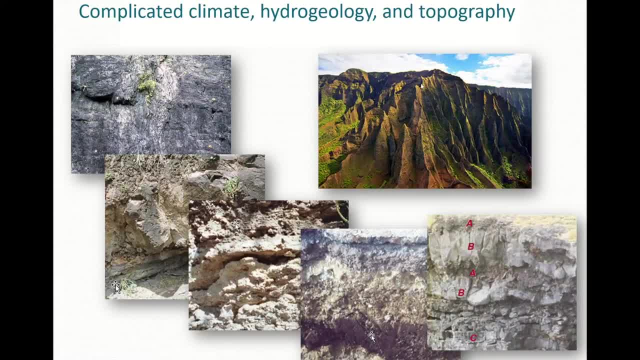 Aquifer are very Or ground surface are very steep And this area is very difficult to access And there is no data available here. So hydrogeology is very complicated by the lack of data And suitability of models to deal with that. 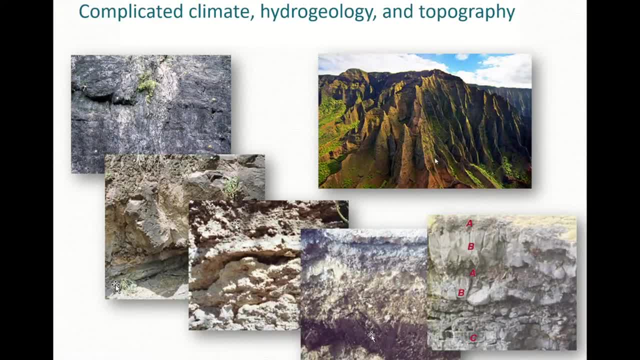 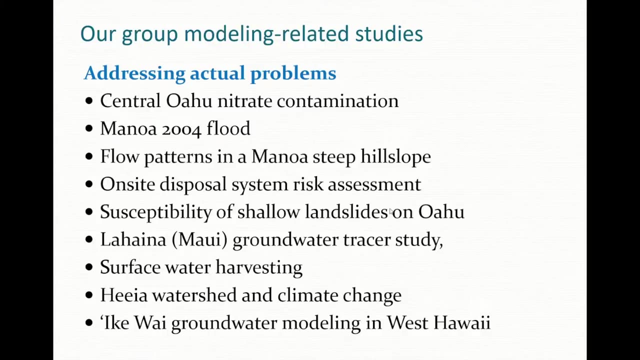 For example, models cannot, For sediment cannot work, for, you know, highly steep area like this, The limits are like 25%, While we have, you know, 100% slope. So here is some of the studies We have done over the years. 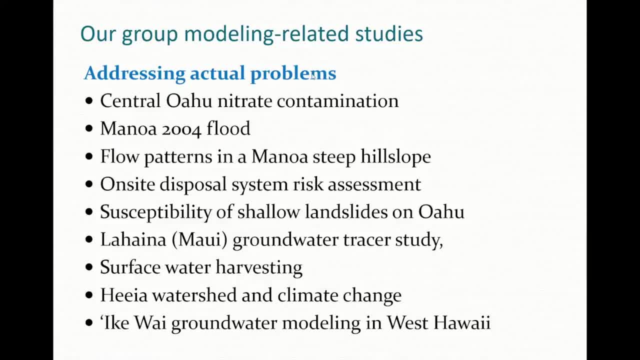 And the objective could be addressing actual problems: Water problems Such as nitrate contamination, Flooding Landslides, Onside disposal systems, Surface water harvesting, Watershed and climate change, And, you know, dealing with specific issues And the big island. 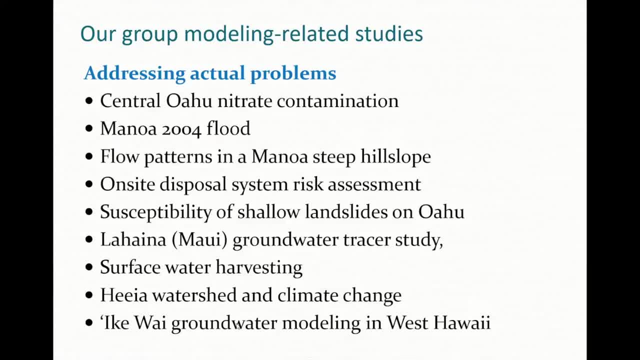 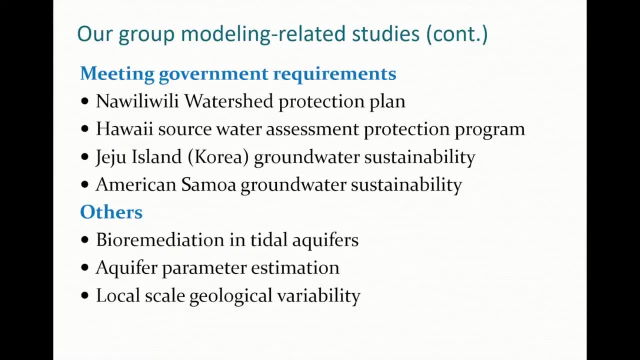 Through water Eqy studies dealing with water availability And understanding of the systems. Then also we did some studies to meet government requirements, Such as designing protection plans for watershed And assessing water protection areas. We did some sustainability studies in Korea, Jeju island. 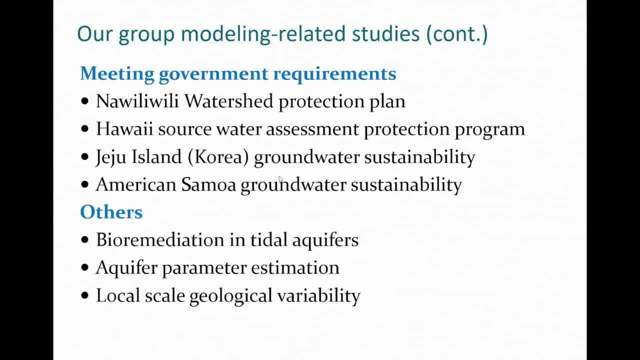 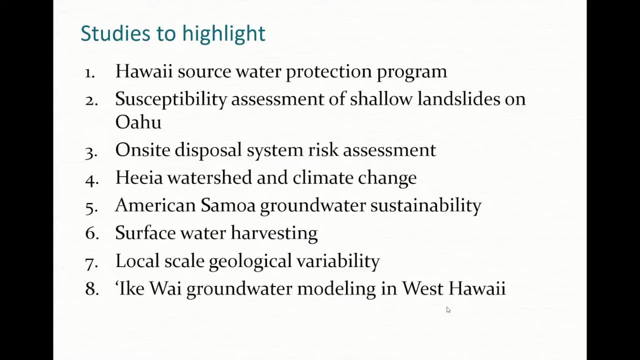 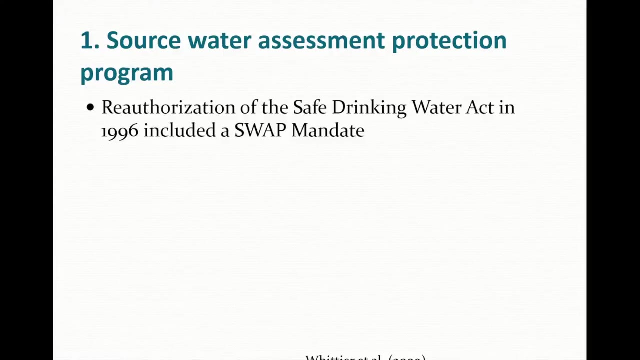 And in American Samoa. There is others which is not falling within these categories, Such as barrier mediation, Aquifer parameter estimation And local scale geological variability. So I will go through these studies very quickly. Okay, Here is number one Is source water assessment protection program. 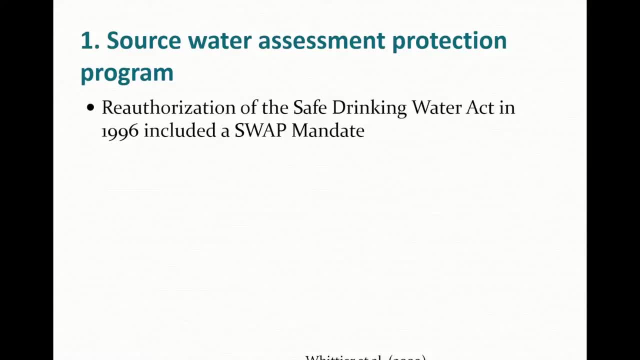 And this is program- was required or mandated by the federal government And that was required through the safe drinking water act, Which was done in 1996.. That included MNS, swap Source water assessment protection program, swap Mandate And this required every state to conduct assessment of public drinking surface and subsurface water sources. 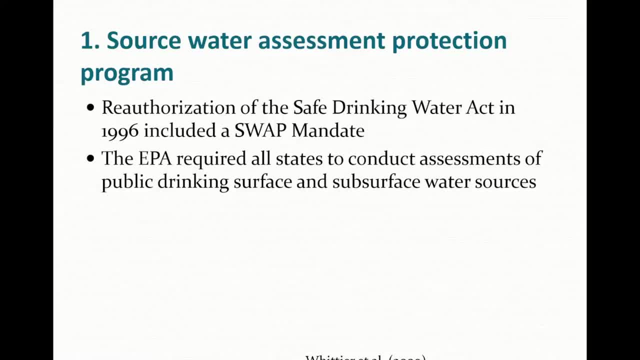 They can be wells, Subsurface Or surface, such as intakes on lakes and reservoirs, And the process include delineating the protection areas, Like, say, around the well, And assess potential contamination activities. Identify all potential sources: Could be actual or existing sources. 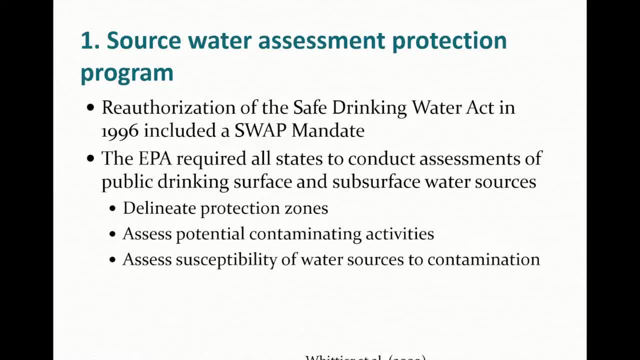 If they have the potential to leak, Such as gas stations, Factories, Military bases, Agriculture, Etc. Then estimate the risk for each source To identify the relative risk- High risk, Low risk- For each individual source. Here is the result. 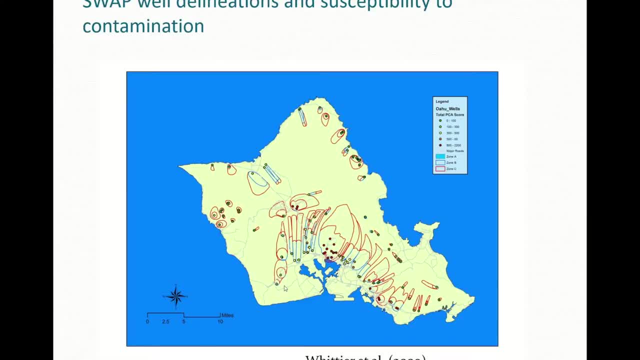 So we can see here- This is for the island of Oahu- Each well is a small circle there. Then we use the travel time criteria And the blue Reflects two year travel time. So any chemical would reach the well within two years. 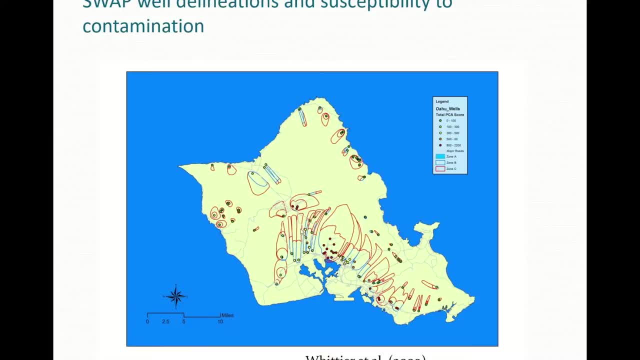 If it was in the blue area here, The red is for ten years. It will reach the well in less than ten years Within the red. So this is how the water source is protected. So we have enough warming time And can do something about it. 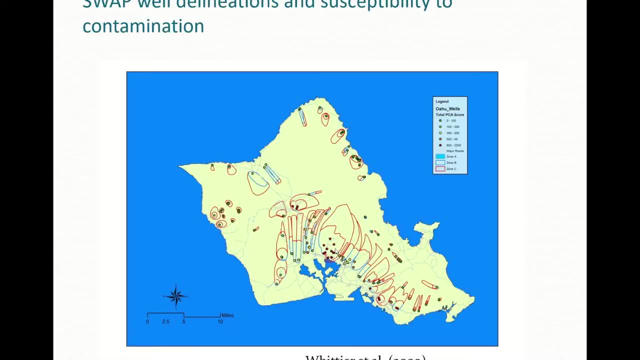 And then the risk is given by the color of the wells: Red, high risk, Blue or green is less risk. And here is the relative values for that. So you can identify the risk And basically see in your planning. That's important to know. 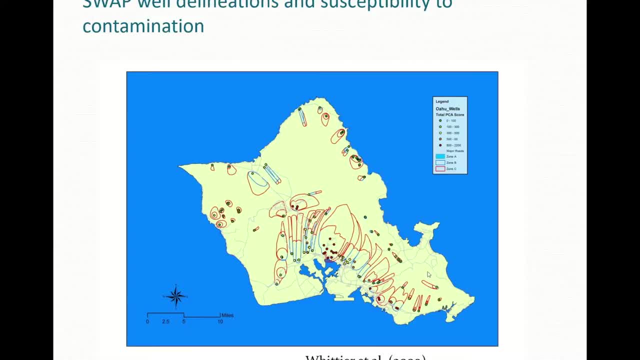 So the objective was just to predict these maps, To create these maps, But actual protection is not Like, for example, I know there is sources of contamination But I cannot do anything about it. But the county of Maui actually used our results. 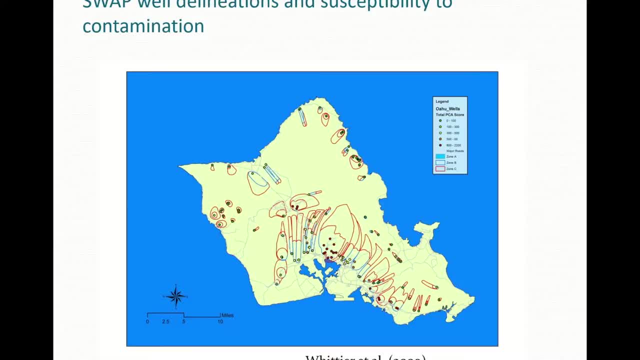 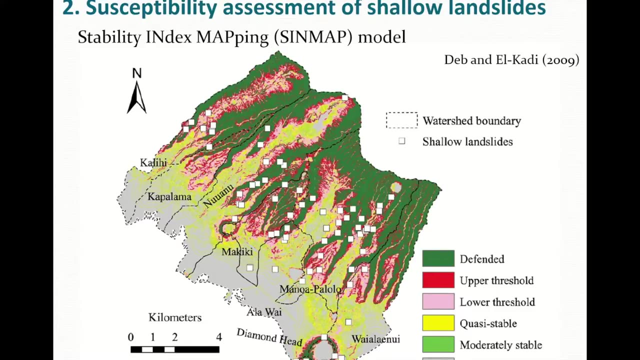 For permitting. So like if you want to have, You know, built a gas station Within the area, They would say no, Because this is not allowed. The second project here Has to do with risk assessment of shallow landslide. What we did, 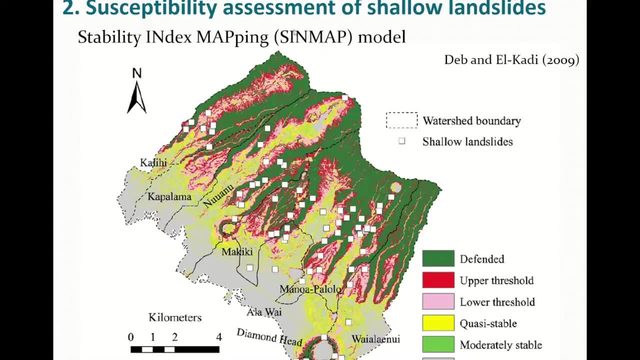 Was to use a model called Stability index mapping, Or abbreviated as sin map, Combined with hydrological information To do To create these maps here, So that would include rainfall Or weather information. That will include the land cover And the soil type. 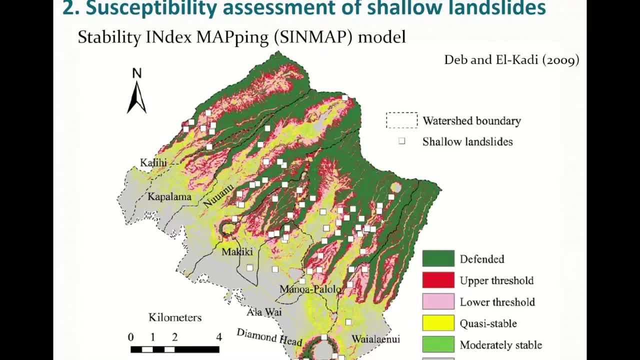 And slope, And what we find out Was to identify the zones Fire risk Defined here as a green- And I don't know why they call it defended And less risk As we go down here Until it is stable, And we tested the validity of results. 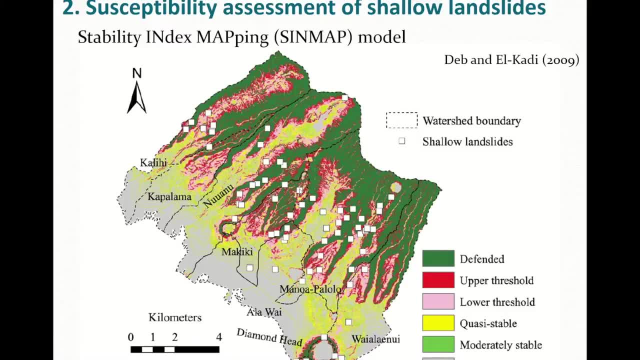 Compared with actual landslides. And these are the squares here, The white squares, And you see the model is reasonable, Most of the actual landslides Falling within the green or red, Some in the yellow here. So that map is useful. 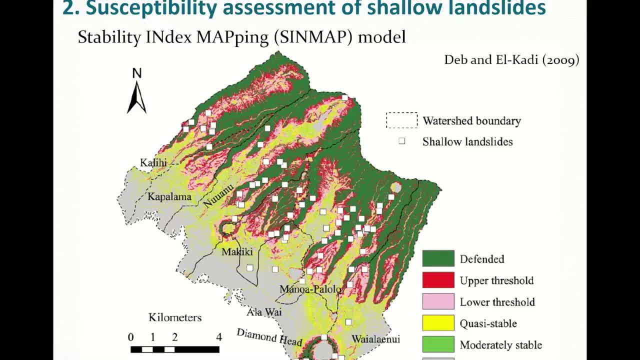 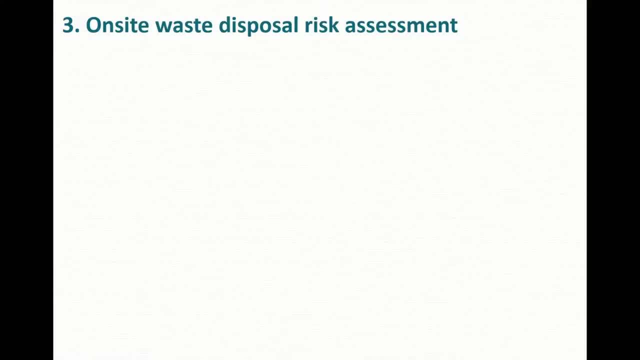 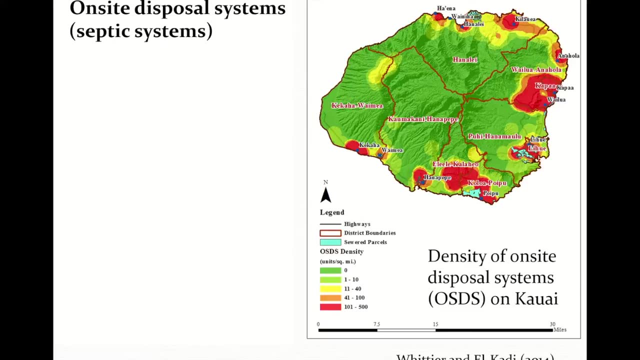 I guess if you are buying a house, That can be useful for your decision making. Number three, On site waste disposal risk assessment. And here is the map For the island of Kauai, And actually you can see here The density of the septic systems. 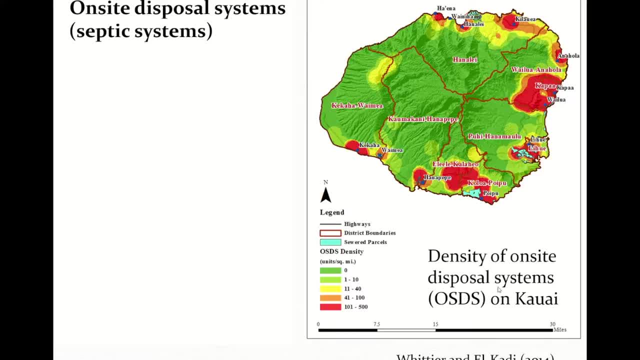 Which are on site disposal systems, Or OSDS, And unfortunately The high density is falling across Or near the shoreline. So you can imagine, You know, for sea level rise That would be very serious problem Because of this And we have really to worry about. 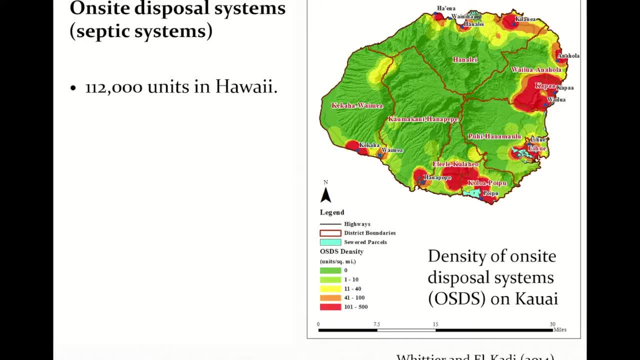 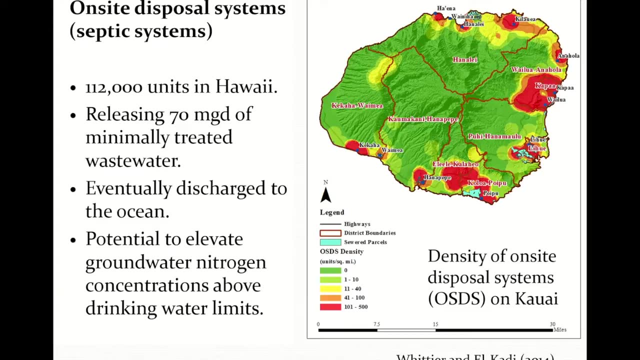 Disposal, Because we have more than 100,000 units In Hawaii And that released 70 million gallons A day Of minimally treated wastewater And that can end up in the ocean And inland. It can increase nitrate concentration. 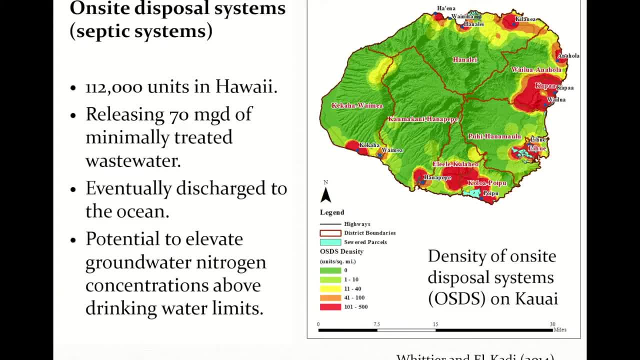 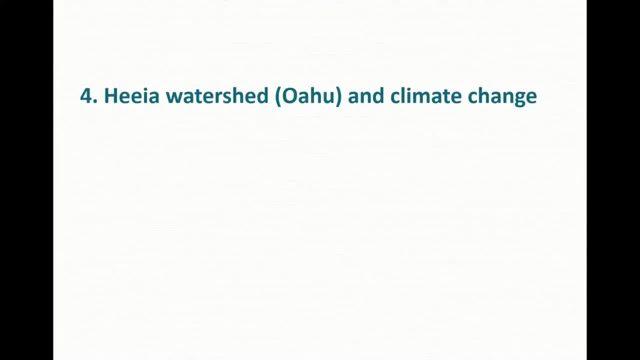 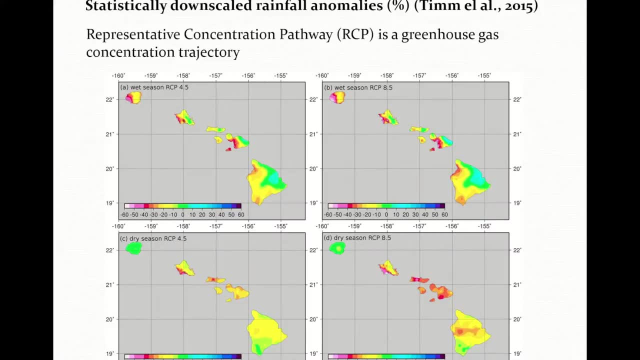 Beyond the acceptable limit. The next one is about A watershed in Oahu Related to climate change And the water project. So here is the climate change maps And we use the statistically downscaled Rainfall calculations And the map shows anomalies. 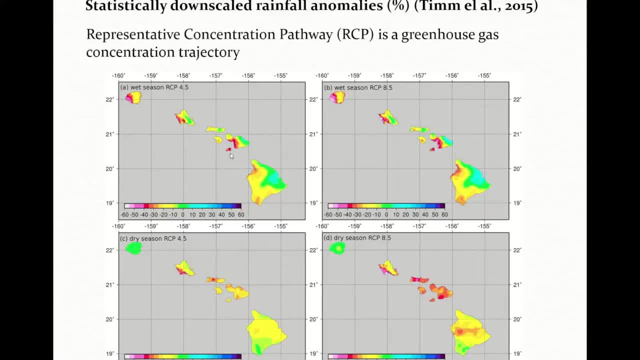 And yellow and red Are decrease in rainfall, Meaning area gets drier, And green and blue Is meaning increase or getting wetter, So we can see the leeward sides Getting drier And the windward side Getting wetter. 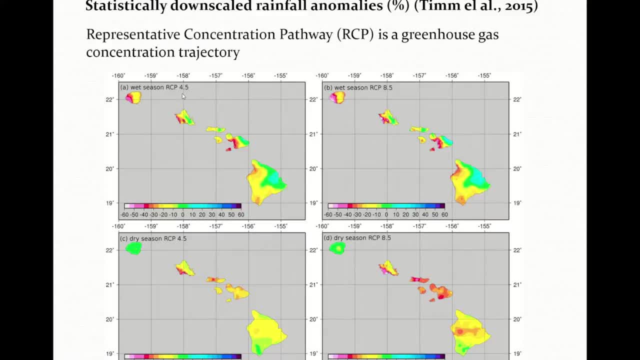 And we use two scenarios: One called RCB 4.5.. Which is representative Concentration pathway, Meaning higher green gases Concentration, And the 8.5. Which is Even higher than 4.5.. So this are for the wet seasons. 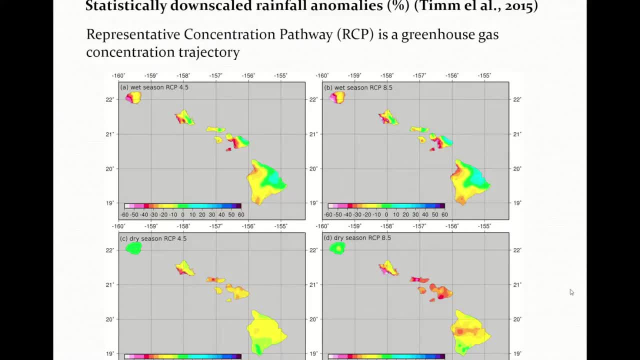 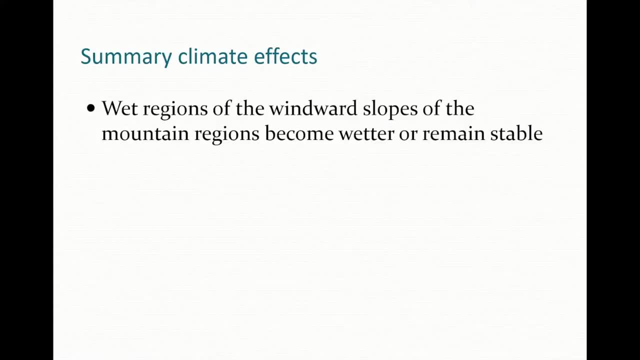 And this are for the dry season And we can see, As I mentioned, The wet regions gets wetter, The dry season gets drier And basically Maui county Looks not so good. It was getting much drier And Oahu has so much changing. 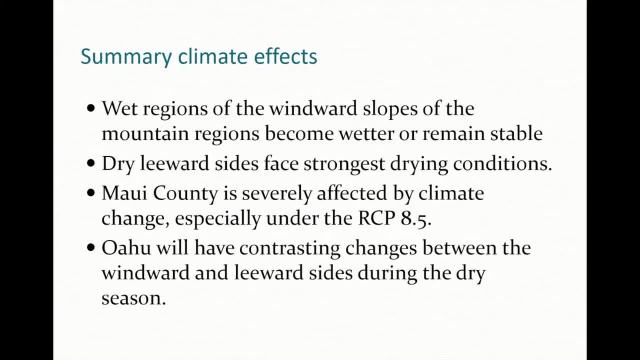 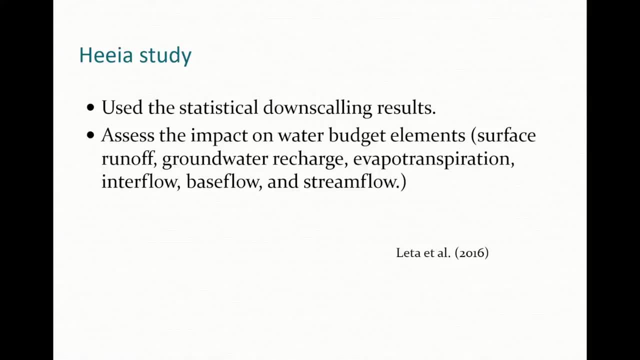 Between drier And wet seasons. So what was the objective Of the yesterday? Basically using the statistical And scaling results To calculate the water budget: Meaning estimate, surface runoff, Ground water, recharge, Evapotranspiration, Interflow, Baseflow. 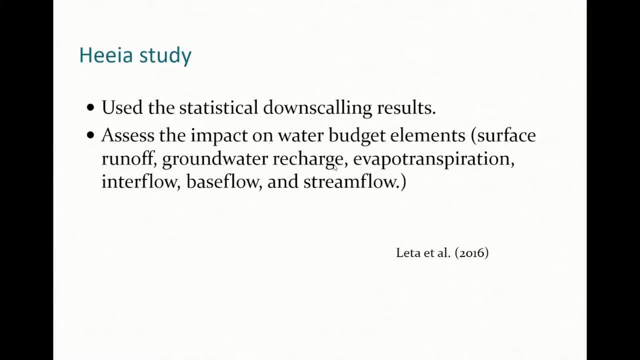 And streamflow. So water falls on the ground Will evaporate And basically that's elements Reflect surface runoff, Ground water recharge, Which is important to assess Ground water sources And flow based flow And up in the streams As streamflow. 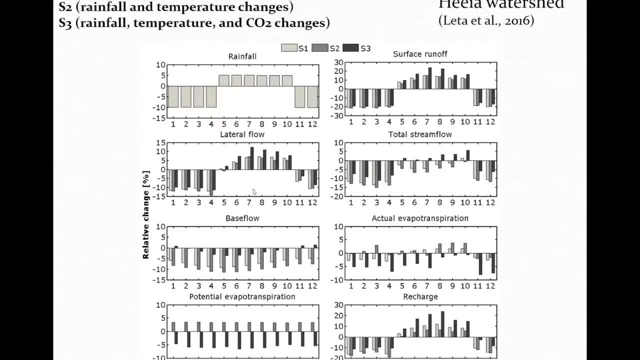 So here is the example Of the results. So here is the change in rainfall- Wetter Dry. Then, based on the changes, We can see how surface runoff Will change. Again, this is increase In surface runoff And here is decrease in surface runoff. 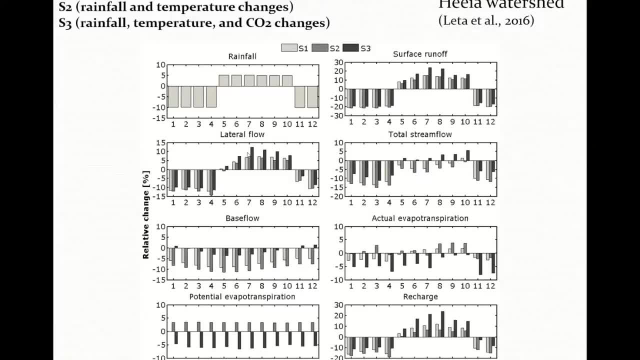 Same for lateral flow, Which is flow from the ground Above the water table, And this is The total streamflow. Here is the baseflow, Which is the flow Below the water table. This is actual evapotranspiration And this is potential evapotranspiration. 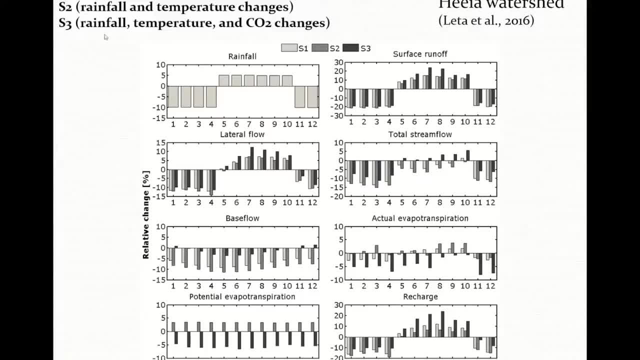 The recharge And we consider different cases, Like here, Rainfall change, only Rainfall and temperature change, And rainfall, temperature And CO2 change. Is more realistic To consider all the three variables Because there is inter correlation Or cross correlation between them. 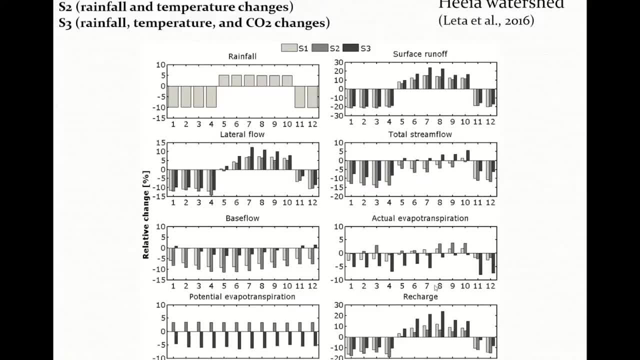 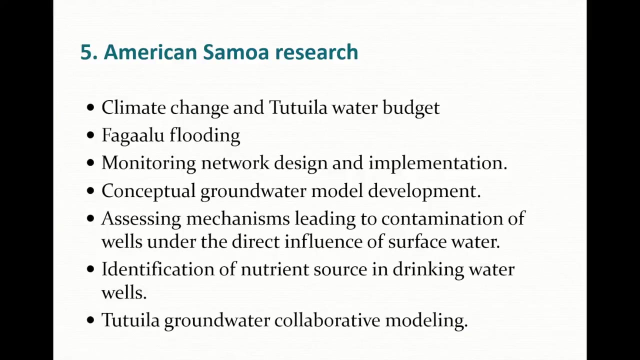 So this is good For planning and management resources. For example, You can address flooding. here You can access for recharge. You know future needs For drying conditions For potential Basically shortages For American And so on. We did number of studies. 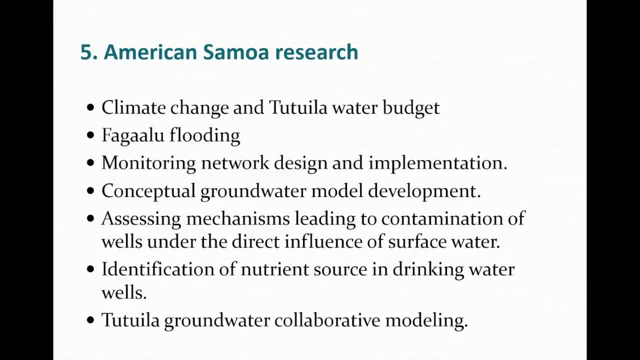 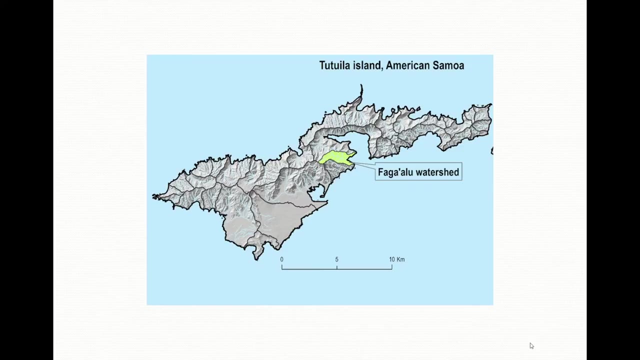 Including restoring monitoring station For weather And for stream Flows. Then did some modeling And assist contamination To wells, Find out which sources of contamination Are more serious. Then did some collaborative Modeling With agencies there. Here is some examples. 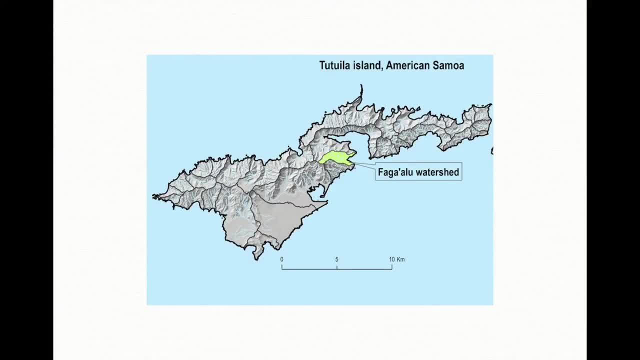 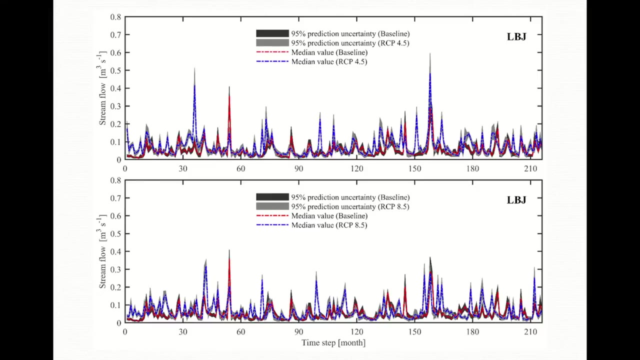 Just to study Flooding And watershed Which is shown in green here Over in Tutuwila Island And The objective was to study How climate change Can affect the stream flow. So the red here Shows you the medium value. 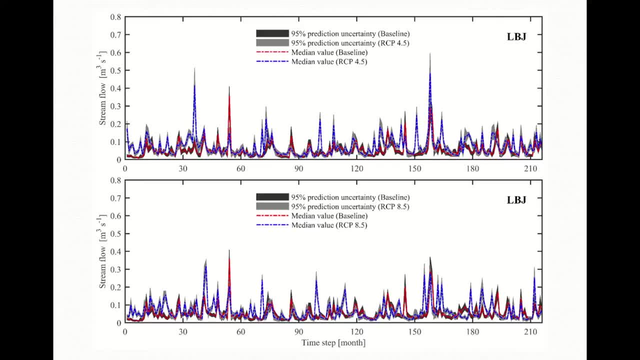 For baseline, Which is the current, Then the blue Is generated Based on climate change, And this is for RCP 4.5.. Here is the same results For RCP 4.8.5.. The conclusion: 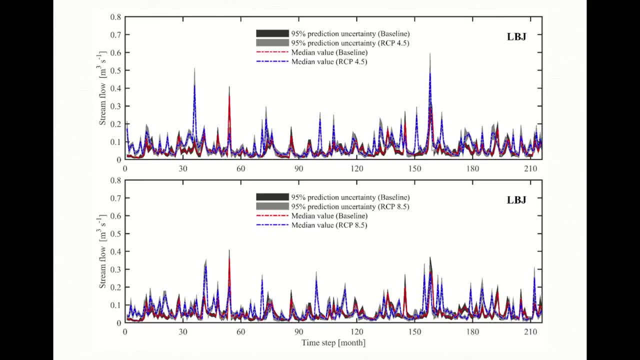 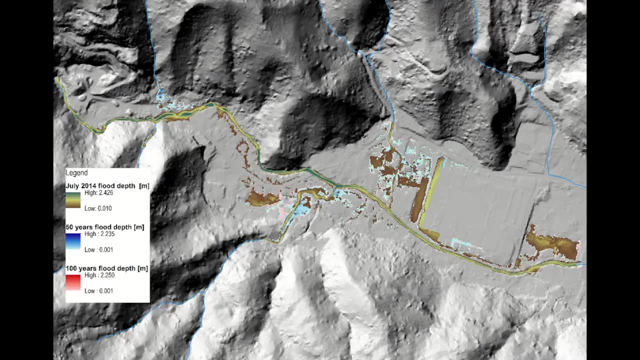 Is that, with peaks Is getting higher And the hydrograph Is getting sooner, Closer or moving, Shifting to the left, Meaning flooding Could be happening On two sides: On Faga'al, Then here is the flooding. 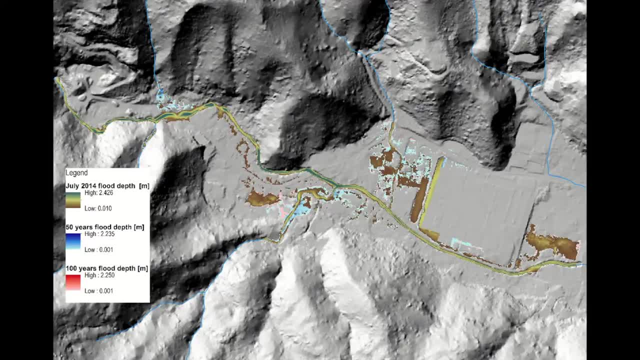 So we Estimated flooding At the lower reach Of the Faga'al stream And you can see This is actual storm That happened in 2014.. And based on our simulations, The peak of the flood Was 2.4 meters. 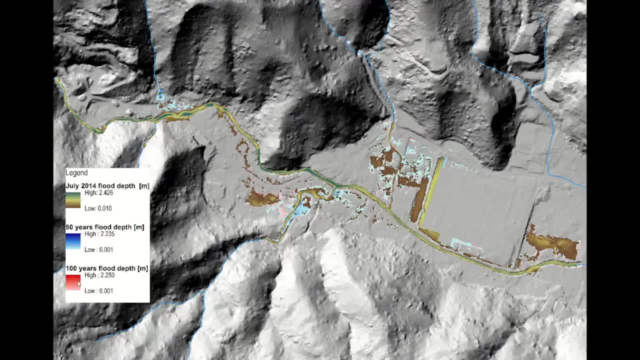 Then we did simulations For 50 year flood And 100 year flood. The brown here Is the actual storm. The blue and red Are the simulations You can see. the peaks Are almost the same. The areas are identical. 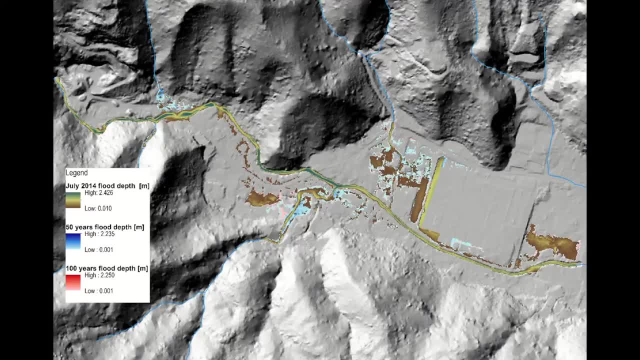 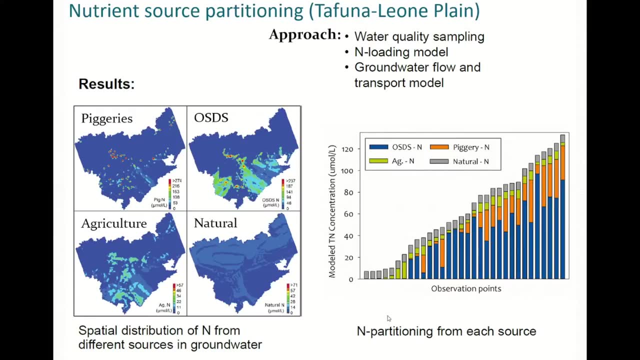 Except some more areas Covered by the flooding. So we believe actually This was very big storm, Close to 100 year flood storm. Then another study On American Samoa Had to do with assessing Sources of contamination Or relative sources of contamination. 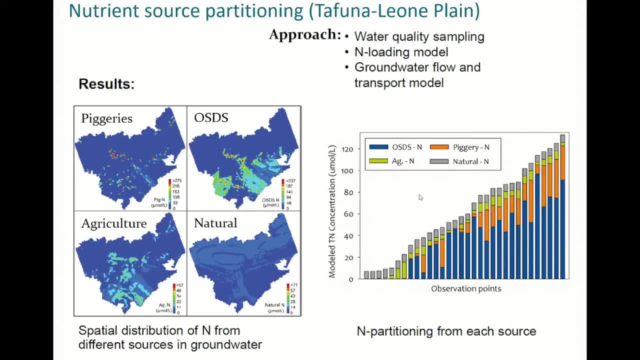 Based on different sources. So American Samoa To Tawila have septic systems, They have agriculture, They have piggeries And there is also Natural contamination, Likely from the Conservation lands. So We found out That OSDS septic system. 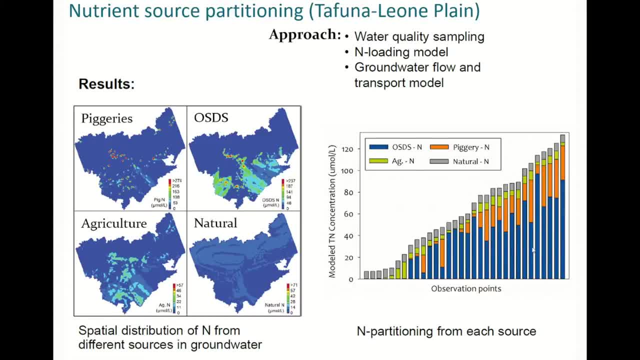 Has the highest risk, That is, the blue color, Followed by piggeries, Then agriculture And finally natural Contamination. Why is this important? Because you can, If you want to reduce The contamination, You start by attacking. 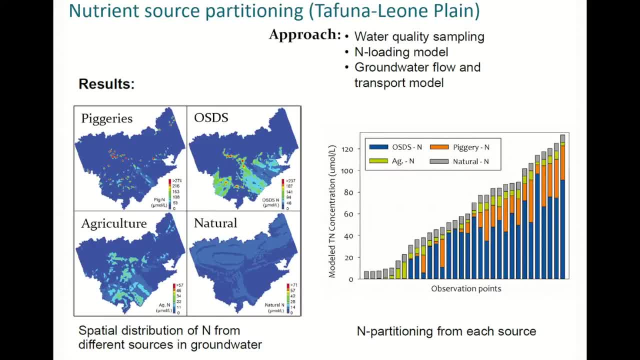 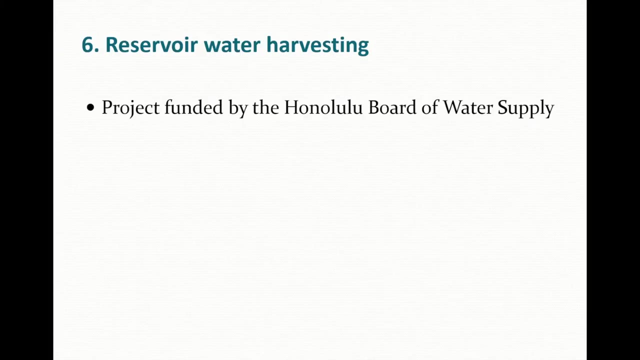 The highest risk, Which is from septic system. This map here Shows the distribution Of contaminants, Because each Or caused by each, Like piggeries here, OSDS, septic systems, Agriculture And natural. Number six Is reservoir water. 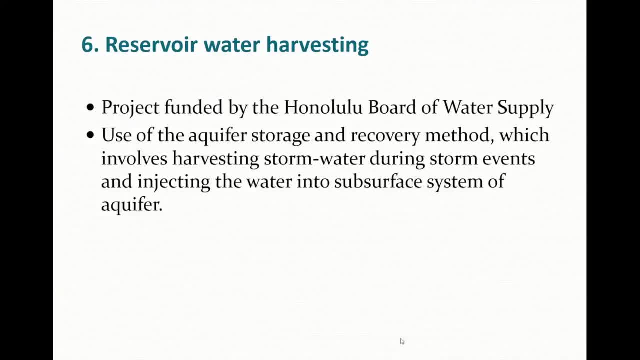 Harvesting, Which is a project Funded by the Border photo supply. The idea is to Collect water from Reservoir, Surface water And injected Into the subsurface. The advantage is that We reduce evaporation From the surface water. 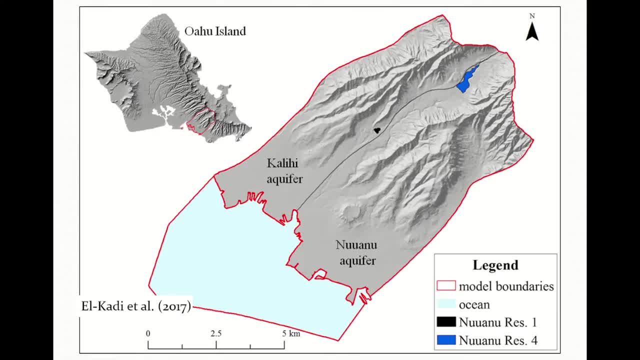 And reduce the chance of contamination- Surface contamination- And also It is consistent With the climate change Because you are collecting And use it in the dry areas. So here is the study sites. This is Kalihi And Nuwano aquifers. 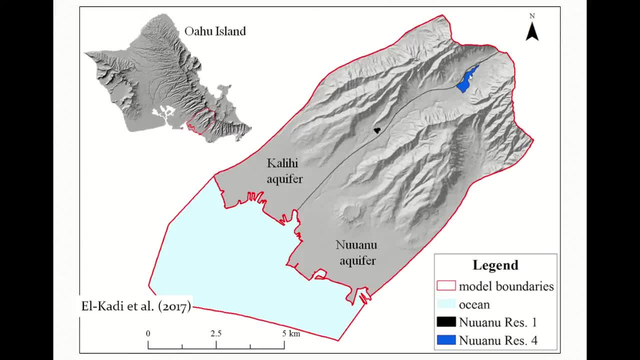 And this is Nuwano number four, Where surface water Will be harvested And injected in this area Near Nuwano number one. So the objective Was to see if it is visible, To collect water And to study how the aquifers 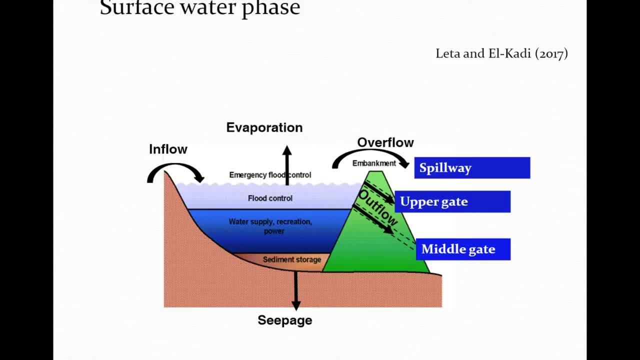 Respond to that. To study The amount to be collected Or harvested, We used a model here For the reservoir And We can basically design The operation mechanism. So we have the water. If it goes above certain level, Go to the spillway. 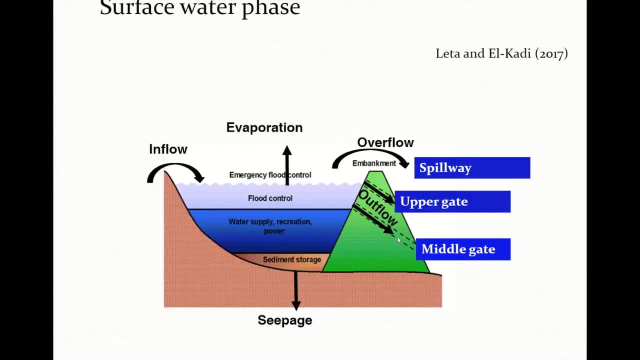 We have gates that can open By different openings To collect surface water And we have to provide, You know, Water spacing for flood control And use water for supplies And protection, Recreation And power. So the idea was to optimize. 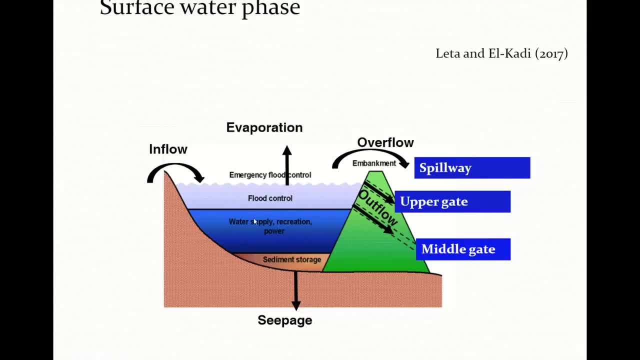 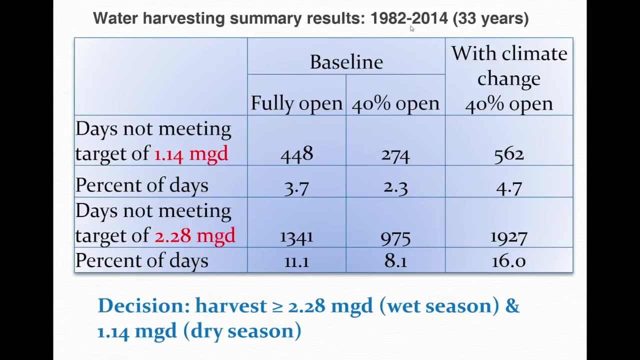 How much you can collect Without violation Of any of these constraints, And we can see also The effect of climate change On these processes. So here is the results. So we have 33 years of data, 1982 and 2014.. 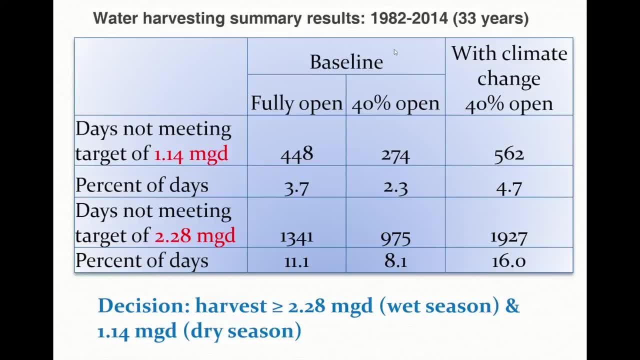 So we use the models To do these different scenarios And estimate That we can collect More than 1 million gallons A day For most of these 33 years, Except 448 days, Which is amount to 3.7%. 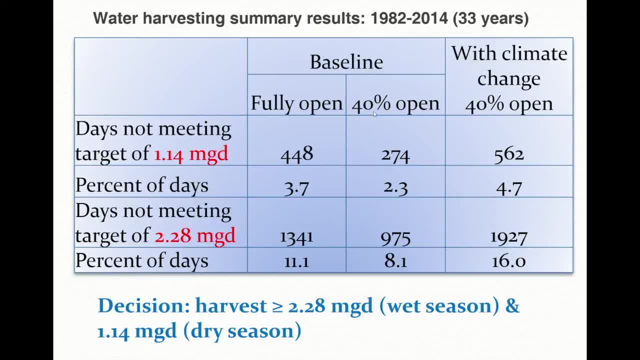 That's if we have the gates fully open. If you open the gates At only 40% For eruption, We only missed 23% Of these 33. Years, That's 274. If we want to collect About more than 2 million gallons. 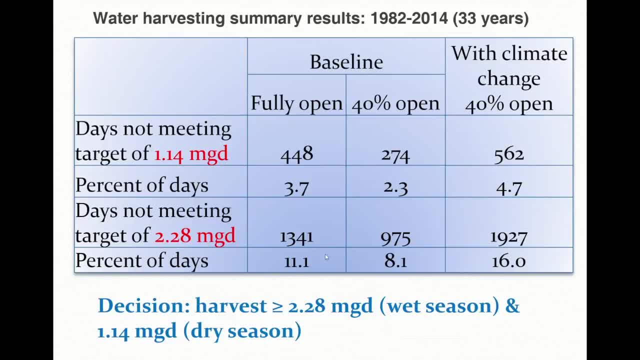 A day. This is the respective numbers. So we lose like 11% of the days And 8% If we open the gates. Here is fully open And here is 40% open For climate change. We have the option. 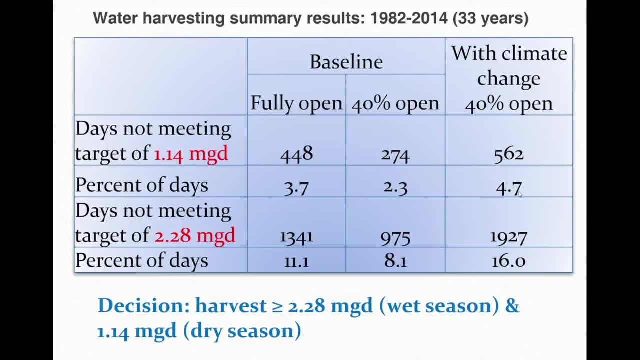 For 40% open And you lose Higher number of days, For More than 1 gallon Million gallons a day And for more than 2 million gallons A day here. Obviously, With climate change, We miss more days. 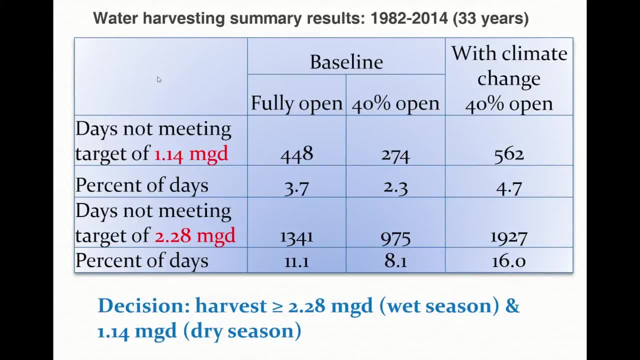 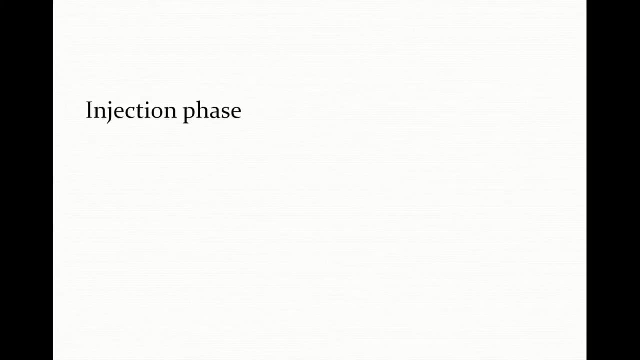 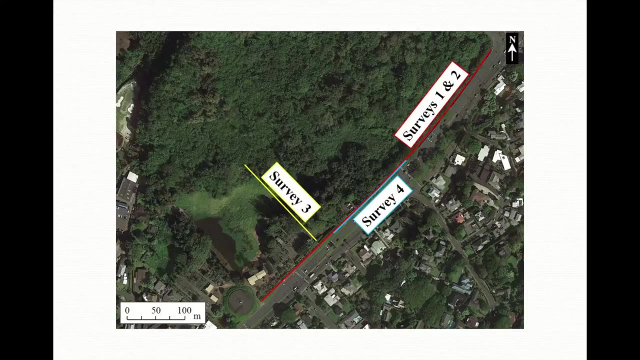 So basically, Very quickly we can collect Between 1 and 2 million gallons With reasonable Strategy. So that was the surface water phase. Injection phase. We did some electrical survey, Thanks to Henrietta, So we did four surveys. 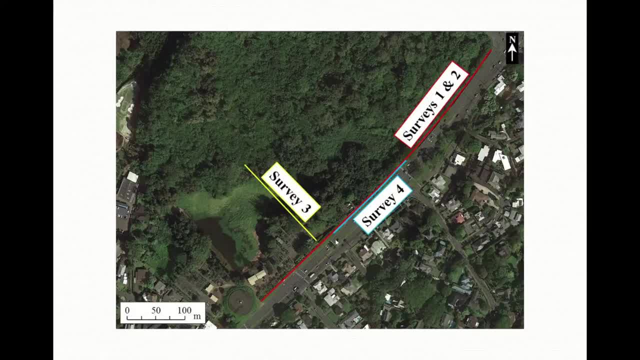 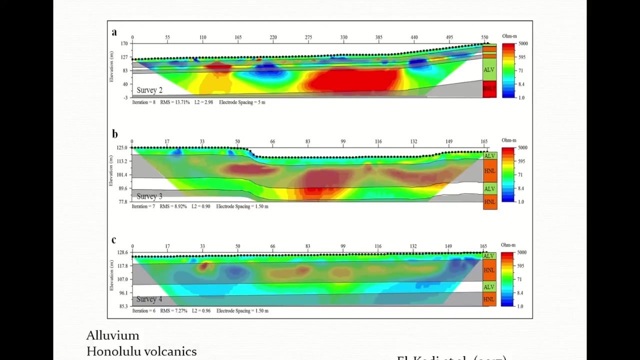 Two along the Highway- This is basically Poly highway- And another Shorter survey, Same location, To get higher resolution. Then one survey Across, like this: The idea was to use Electric resistivity To find the subgeology. 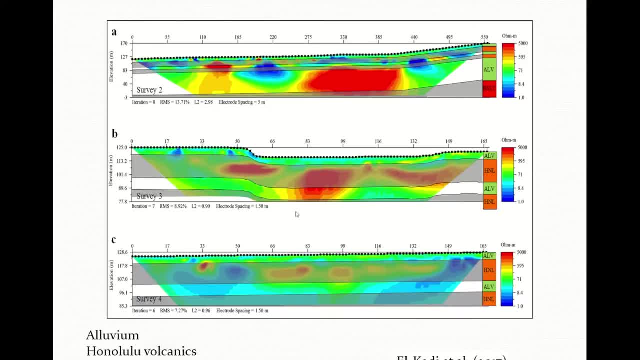 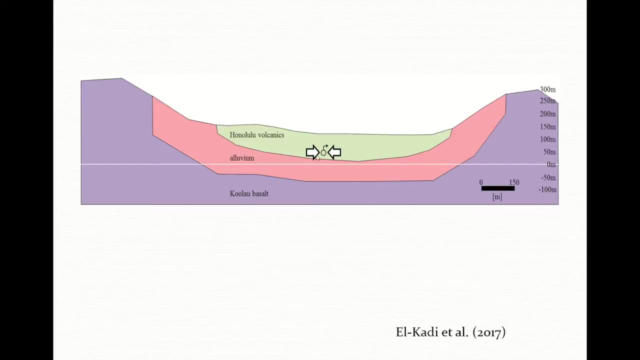 And we identified Olivium Monolulu, Volcanics, Koala And the distribution For the site. So this is idealized Cross section like this And unfortunately We have to inject Above the water table, Which is the white line here. 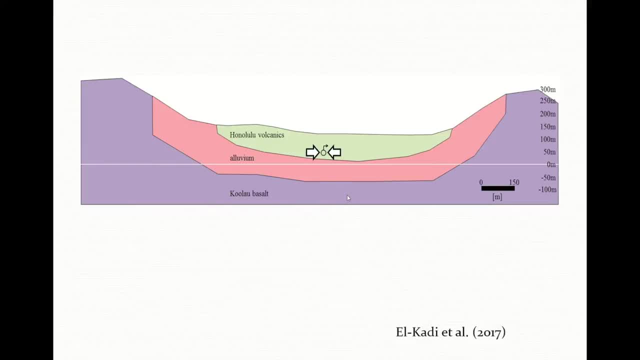 Which would be done In the Honolulu Volcanics, Because we cannot really inject Below the water. It should be nicer to inject, But this is not allowed. So the idea was to simulate The injection process To make sure that we can. 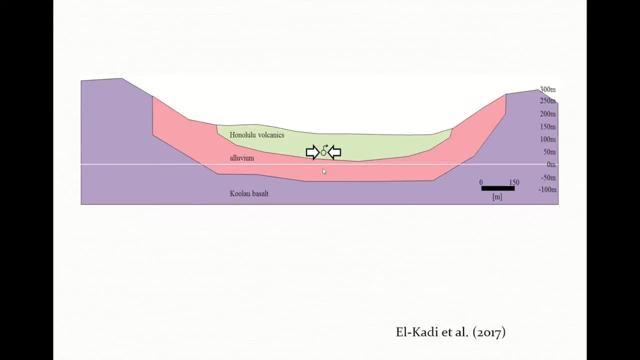 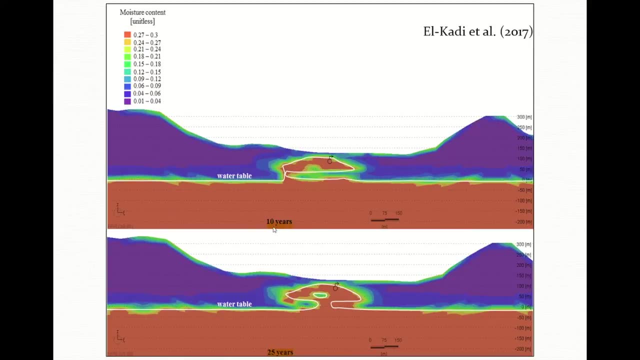 Have enough room Not to connect To the water table Or flood the ground. And here is the result: This is after 10 years And this is after 25 years. You can see it is still okay, But it is very close to being connected. 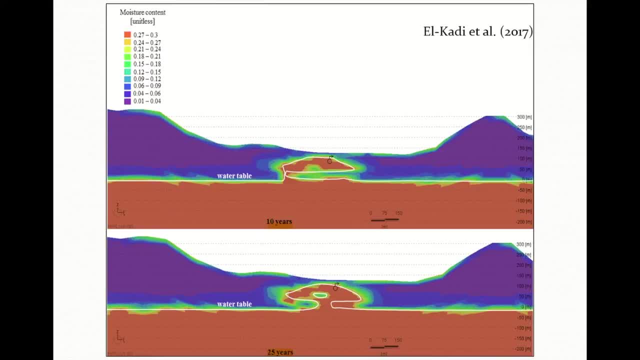 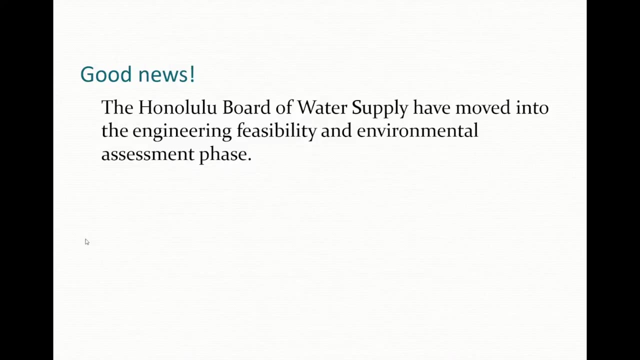 With the subsurface, With the saturated zone At the water table. So we recommended To either reduce the injection Or distribute Over a number of wells, Over the head, And the good news is actually The boat for the supply. 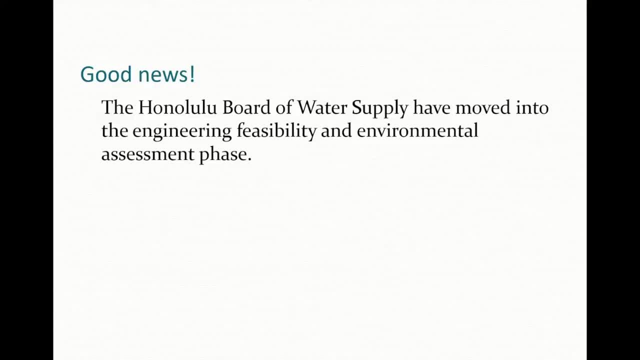 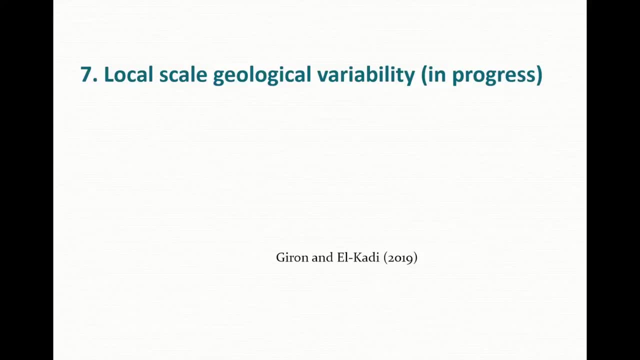 Is planning to do the project And they started already The engineering approach. The next one Is local scale Geological variability, Which was done with One of the REU students, Which is just In the past summer. So let us say 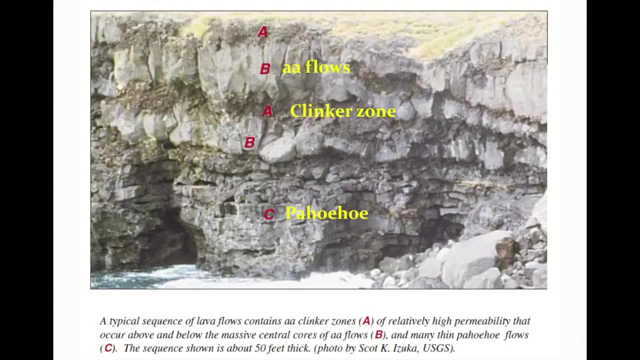 This is, You know, Basalt formation, Which is number of flows, And that can range by Clanker zones, Which are highly compacted And are flows. So this is basically The real life And we can digitize it. 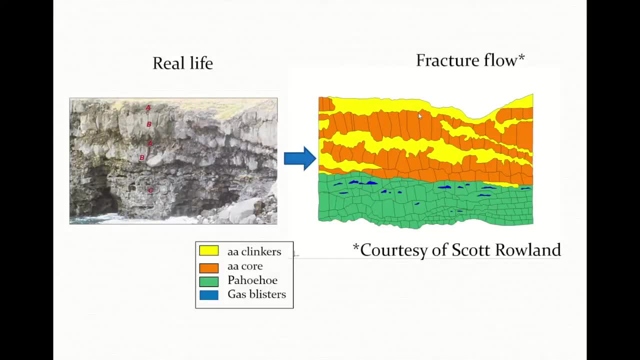 Like this And see the fractures here, And thanks to Scott Who made this map And digitized for us. So this is the real life And this is our conceptual model Of that real life. So water can move Faster in the fractures. 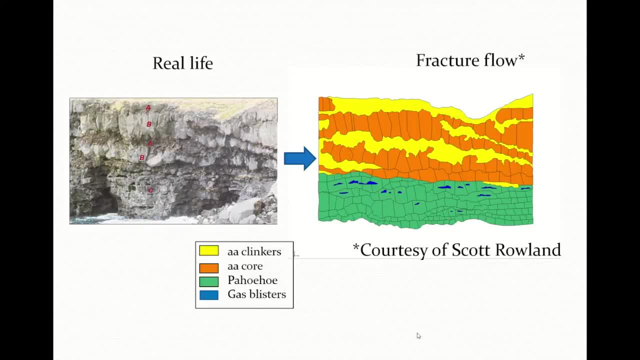 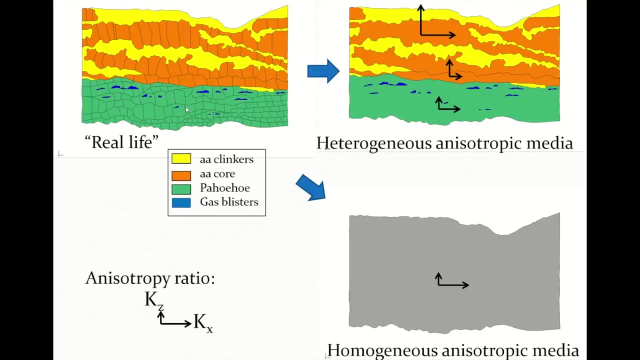 And basically Could be also flowing Between the fractures And the matrix. So the objective was, If we can approximate Further, approximate this As porous material. So basically no fractures. This is all porous material And Of different conductivities. 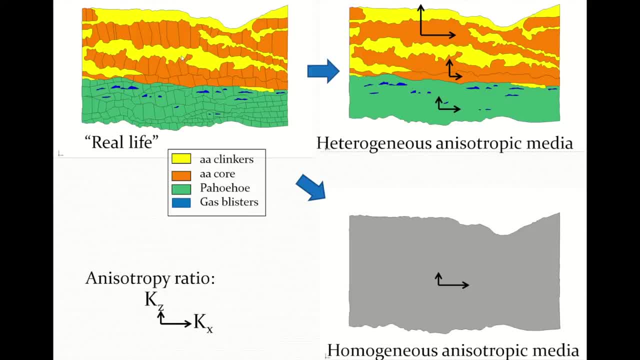 Or we call it Effective conductivities. And even if you can go further And use only one material Rather than one, two, three materials Here, And the arrows give you the conductivities And the vertical and horizontal That can be different. 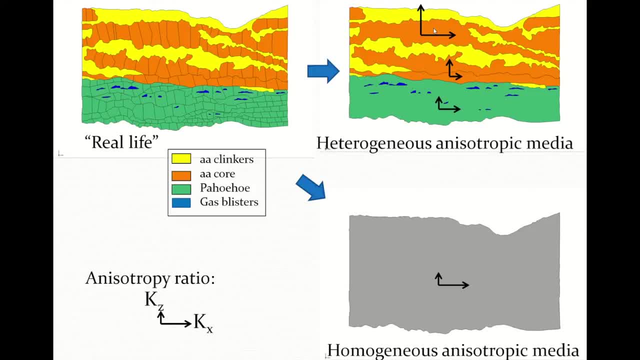 An isotropic feature, So this is heterogeneous. This is homogeneous Meaning the same conductivity everywhere, But it can change between Vertical and horizontal. So again, the objective is We can replace this real system With this approximate system, Or by using effective 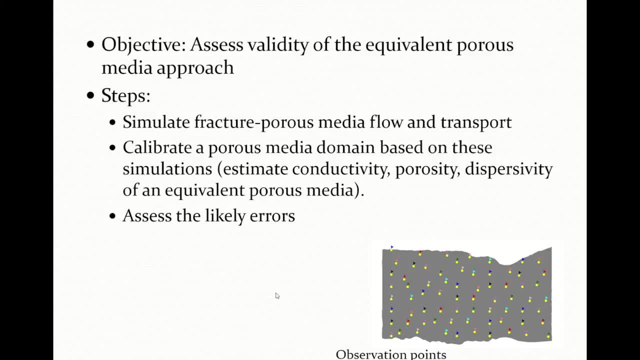 Conductivity. So here it is The validity Of the coherent material approach Which is replace the fractures With the porous material system. So first We simulate the fracture porous media For water flow and transport. Second, Calibrate equivalent system. 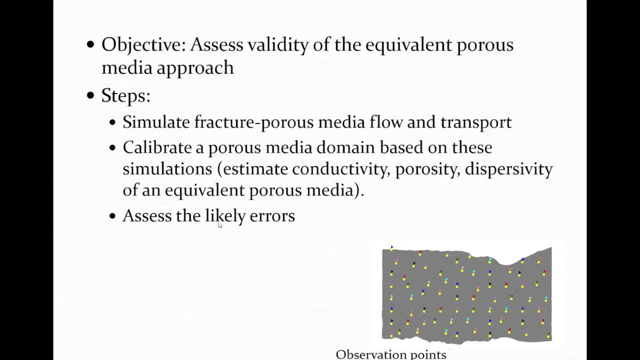 By trying to match Whatever result we get from here And assess the likely error- Error expected Or error- because you don't expect The equivalence to be 100% Correct, And here is monitoring points. So we try to match Our simulations. 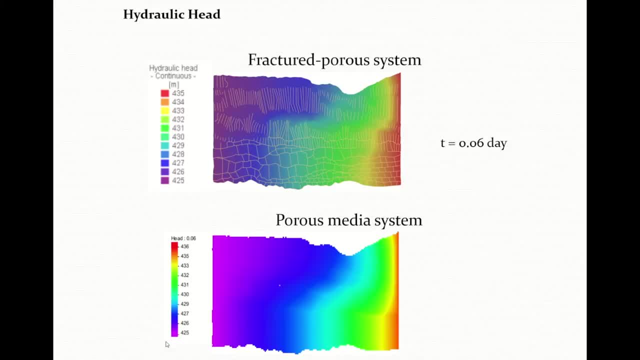 At all of these points. So here are the results. So here is the hydraulic head At different Locations And this is the fracture porous system, The real one, And this is the equivalent one, And you can see the image. Where is high is high. 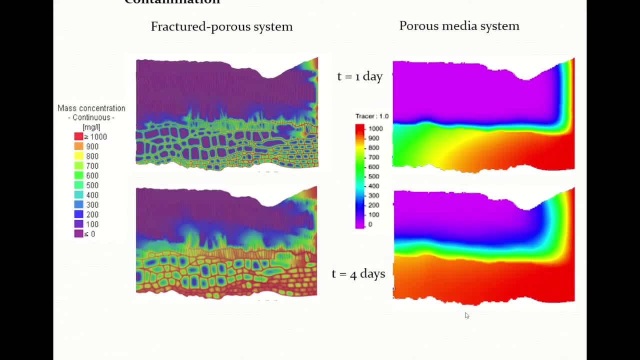 And where is low is low. This is at certain time, And here is the contamination Going from the side. We can see the effect of fracture flow. We can see preferential flow, Where the contaminant move faster Through the fracture. 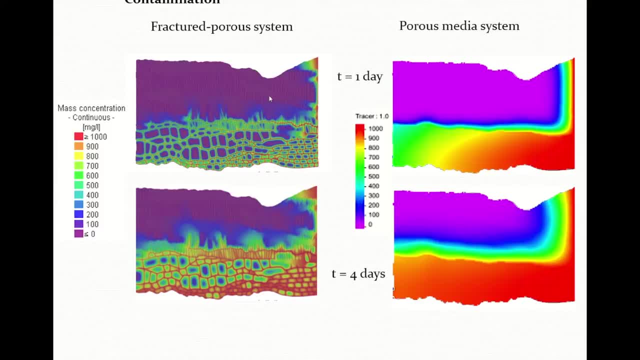 Slower within or between. So this is after one day And this is equivalent porous media. We can see the same trend. You know, high is high And low is low. But obviously there is huge errors. For example, here is no contamination. 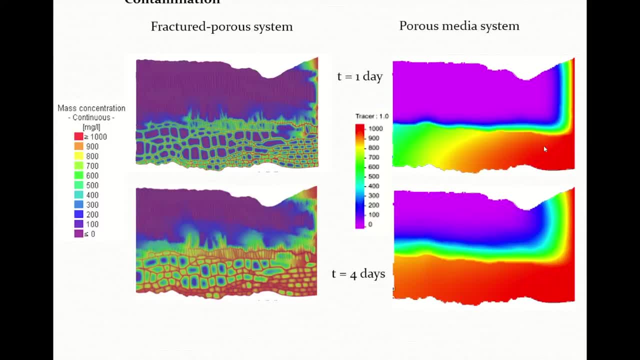 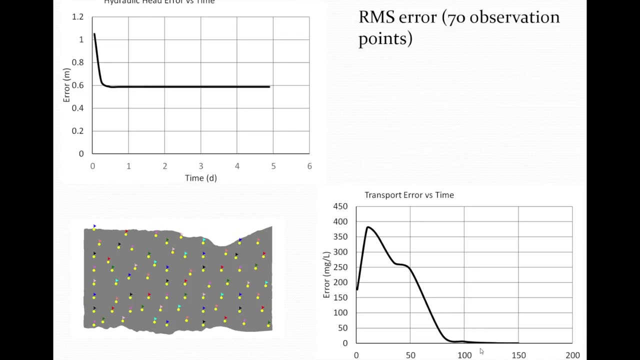 You know, Between the fracture And actually the model here. It is high concentration And it can change with time. This is after four days For the porous Fracture- porous And equivalent one, And we found out the error. 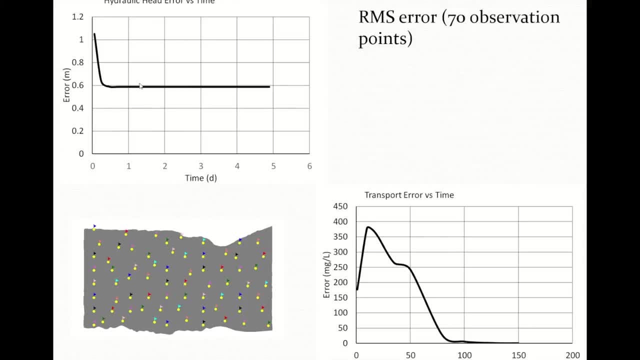 Gets very small And even smaller very quickly As we reach steady state. For hydraulic head, However, the error is significant For contamination, So only after 100 days X is accepted. So the conclusion: We can use porous media Assumption to model flow. 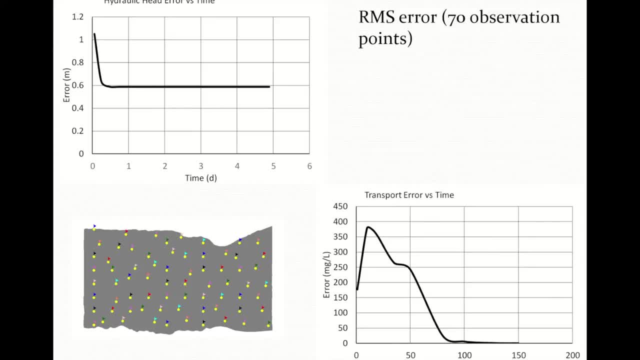 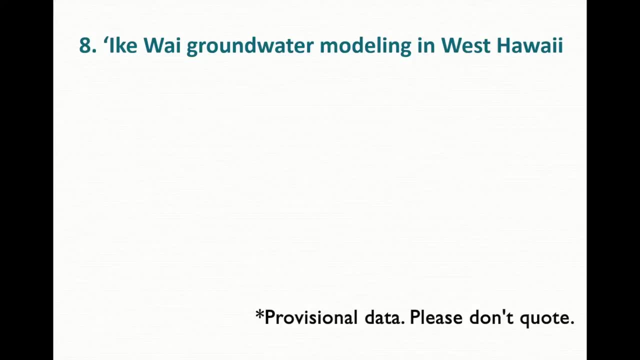 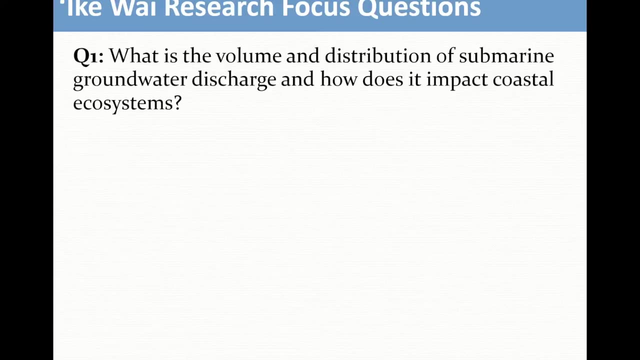 Water flow But we cannot really do it For transport. The last project Is the EQI modeling. We have been doing it In West Hawaii And the objective Of EQI Is to study Underwater discharge And how does it impact. 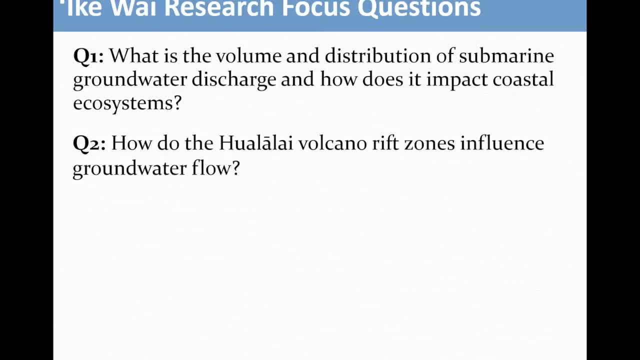 The coastal ecosystems, Then How could we, You know, study? Or what is the impact Of the rift zones On ground water flow For the Hawaii Volcanoes Aqua area, Then what is the source Of water? So, basically, study the amount. 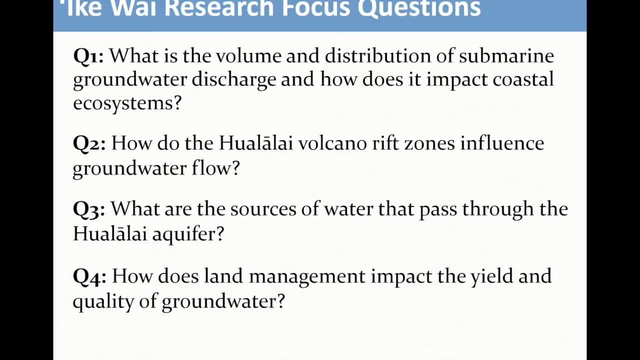 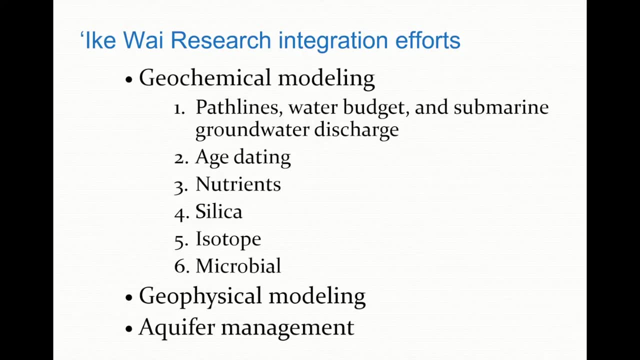 For water As it goes through the ocean. Then, finally, How this flows Affects the water quality And the specific Yield of aquifers. So just for managing The sources, The resource, So we will integrate Our numerical models. 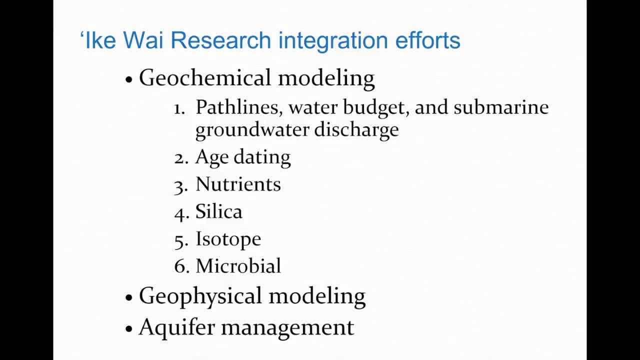 With geochemical modeling, Such as the bath lines, Water budget, Water field data collection, And we use this information To calibrate and validate Our models And for age dating Nutrients like Nitrate, Silica And isotope. 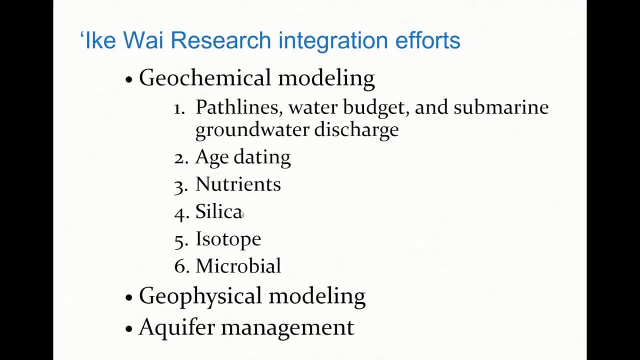 As well as microbial. So, again, all of this information Can be very valuable In calibrating and validating Our models. Another important Is the geological modeling, Where we try to build accurate Geological model For the aquifer And use this information. 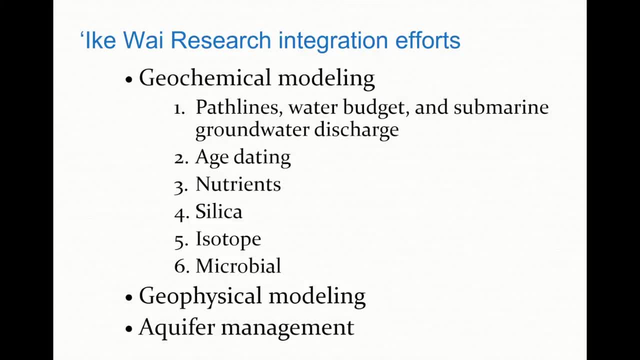 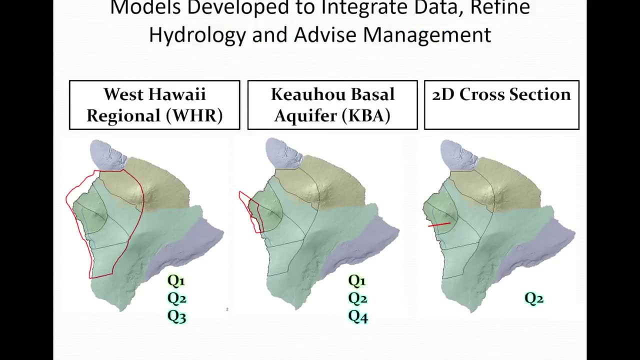 Again for validating, Calibrating and validating our models. Once we are done with this, We use information And the model To do aquifer management, To study water quality And quantifications. So we developed Three models. We call it WHR. 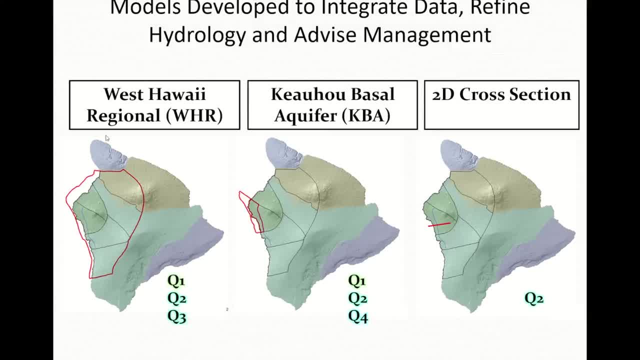 For West Hawaii regional model Covering this large area here, And we have to extend to the ocean So we can study Submarine ground water discharge. And this is used to answer questions One, two and three When two has to do. 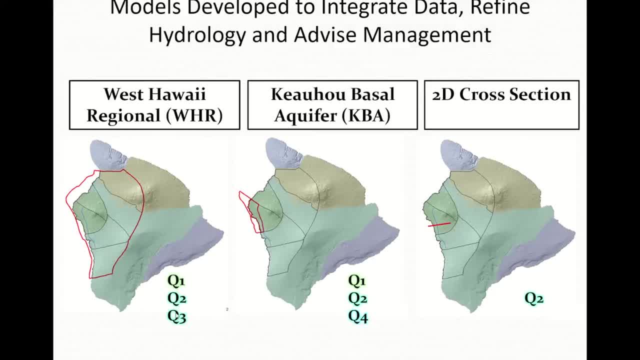 Or when two and three Have to do with water flow And submarine ground water discharge, Then this is covering A smaller area. We call it Keahu And this is used to answer Question one and two: Water flow and pathways. 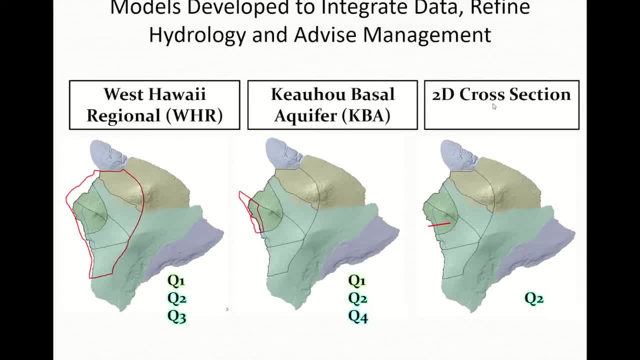 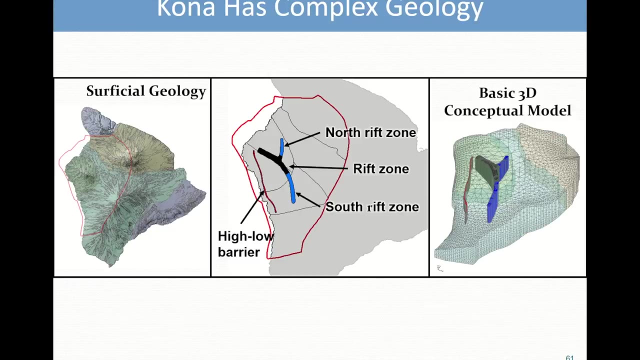 And Q4, which is the management. Then the cross section model Is used to answer Q. You know flow and basically We can integrate it with Available information to build Basically Better Model for flow Bath lines. Then this area is very complex. 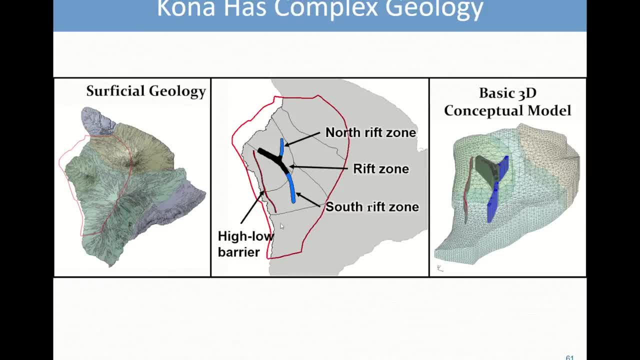 So this is like the large WHR model And you can see here the surface geology: Three volcanoes, Very, very complicated And we don't know really the extent Or the distribution of geological At the greater depth We have. 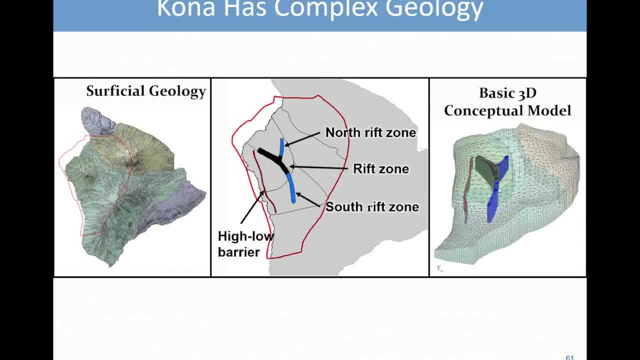 Rift zones. Some of it are not well defined. We don't know, even if, How deep that formation is And we have what we call a barrier: The jump of water level Less than three meters To how much higher, 50 meters or more. 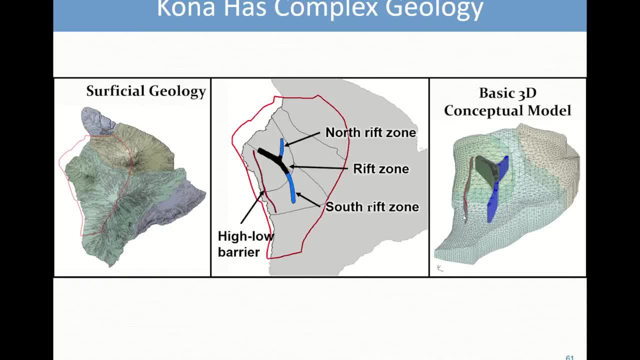 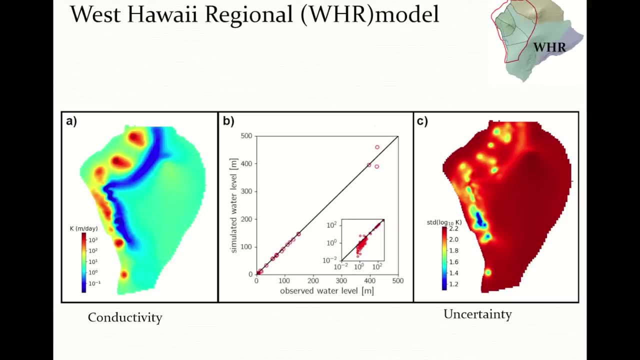 Across from the barrier. The exact reason for the jump Is not well known, So here is some of the results. So this is for the West Hawaii original model, WHR model, And we calibrated the model To try to predict the 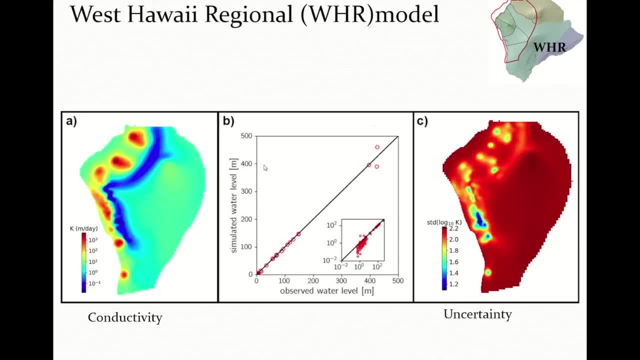 Measurements for Available records. So you see, the calibration Is very good And the model was able to identify The need for low conductivity zones. So here is what we call a barrier, But actually the barrier Should be extending here. Unfortunately, there is not much. 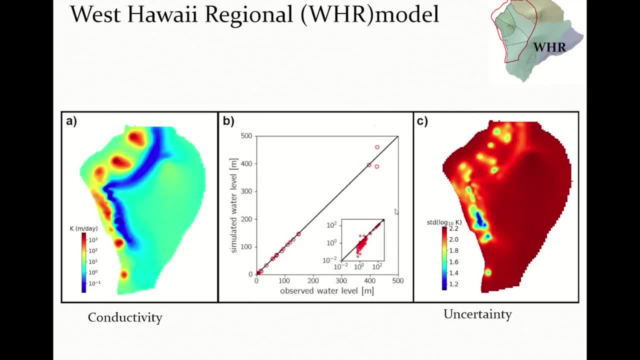 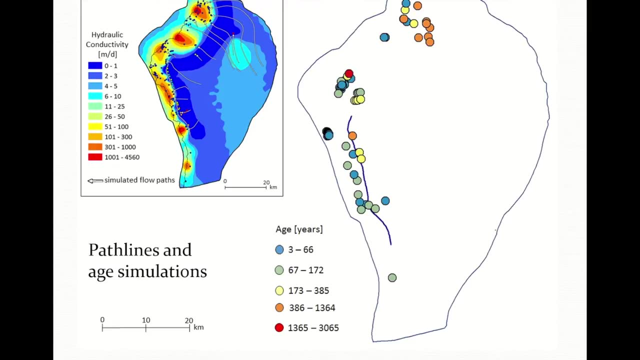 Data available In the high level area Or high elevation area, And you can see uncertainty here, Not very high uncertainty In this area. So this is for information Through geochemical And geophysical research. Then we simulated Age. 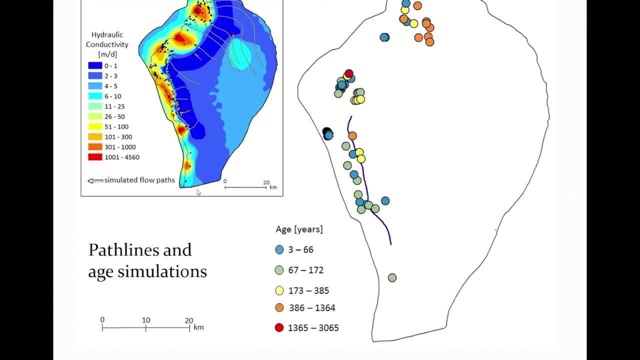 And we found out that, Based on model calibration, This is the hydroconductivity Which I showed in the previous Snap, Excuse me- And the model predicted Much older water In this area than here, And this is supported. 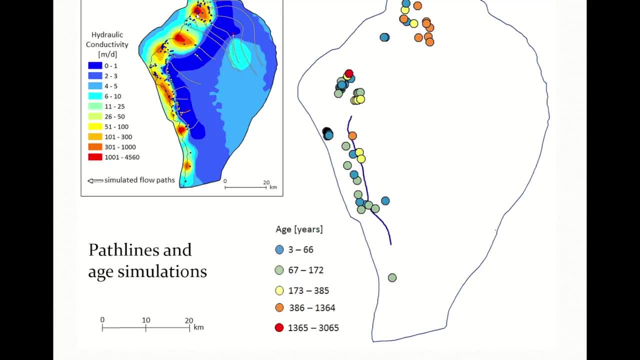 By the simulation Of travel times. Obviously this water is older Because it resembles water That travels long distances here, Compared to here, Which the source is much Closer Or the path lines are shorter, So ages here should be. 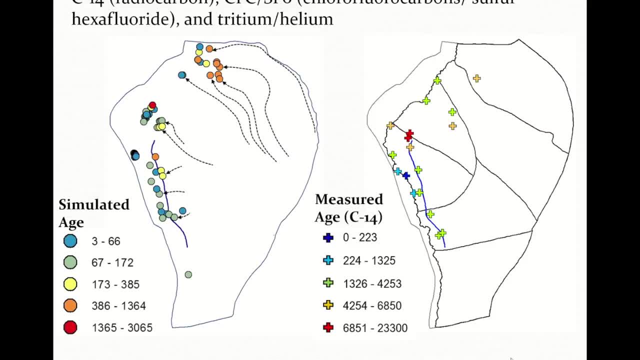 Younger than here. This is all modeling, But to calibrate Our model We have two measurements: C14 CFCs And tritium helium, And this is the simulation I showed in the previous screen. They reasonably match. 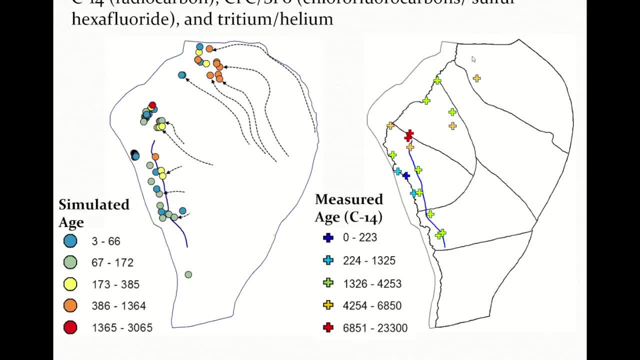 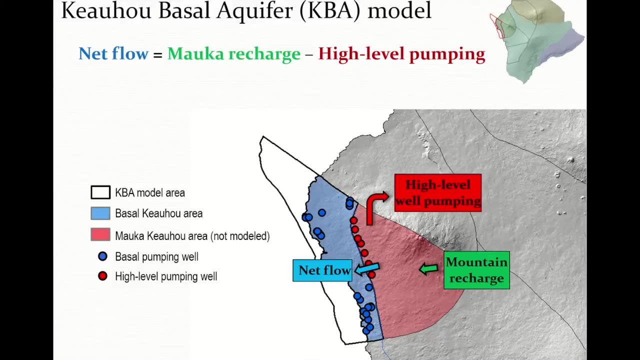 You know The measured C14.. We are still doing some work on that, But low or young And old. This is the third Or the second model, Which is KBA Or KIAHU, Basal aquifer, And this is a simplified model. 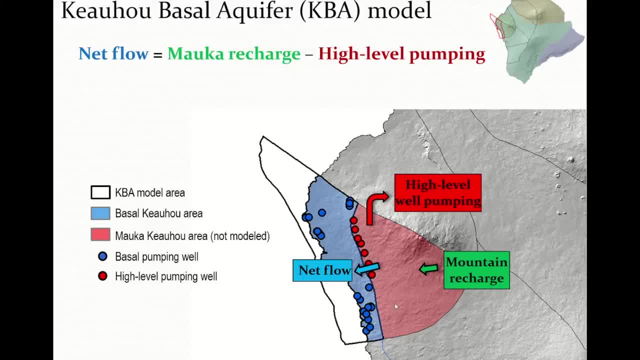 We estimate the net flow Across the barrier here And just to model The area outlined here And basically It is more suitable For managing the sources Below the barrier. So we did not simulate the flow here, We just estimated the net flow. 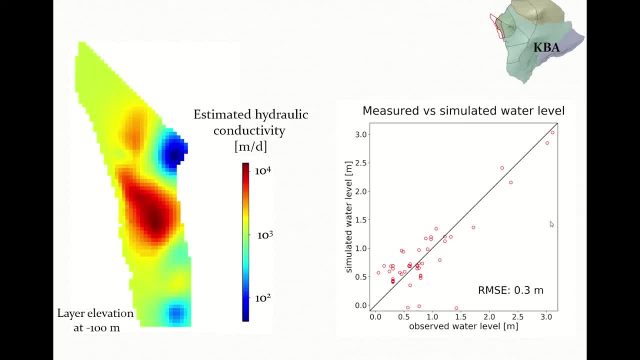 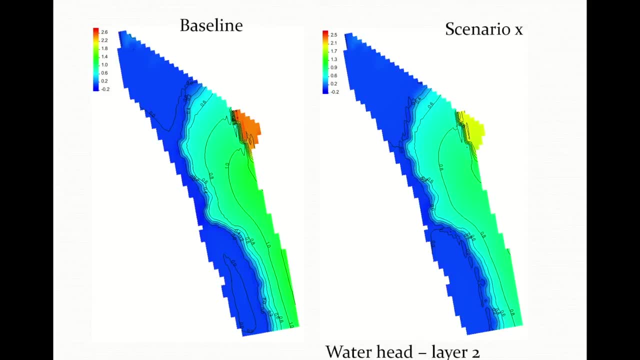 Here And we did the calibration. It matches well, Which gives us the distribution Of hydroconductivity. Then we can do scenarios. This is the baseline Which is current And this is, let us say, Due to climate change Or overuse. 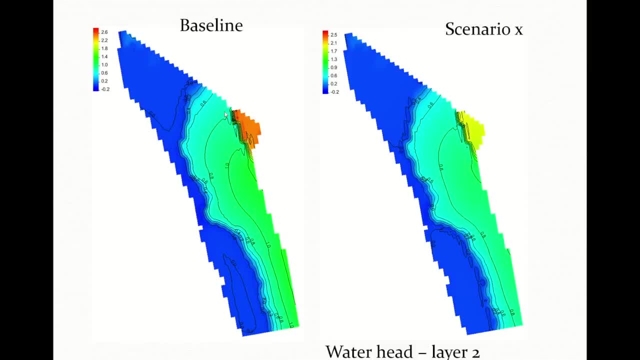 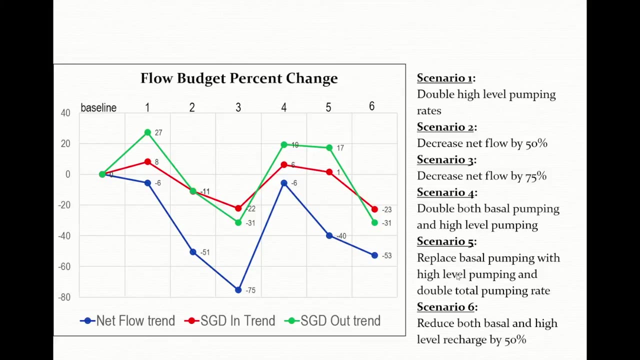 Or things like that. Then we can see decline for water level. This is water level for the baseline, Current Reduction And recharge. There is example for the water budget. We can do different scenarios, Like the blue here Reflects the net flow. 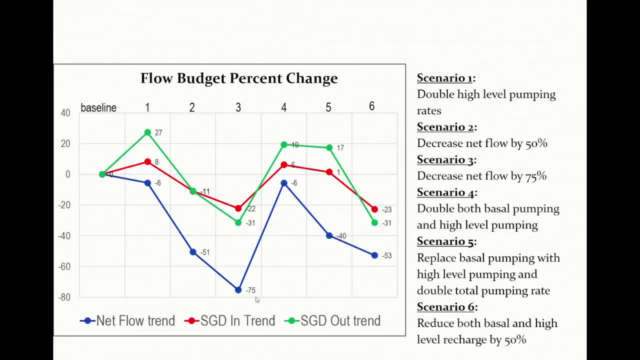 So here, up to minus, This is percentage, Like 75% reduction And We can look at the red Which is SGD Coming into land. So this is from the ocean. We can see Like increase, 8%, decrease. 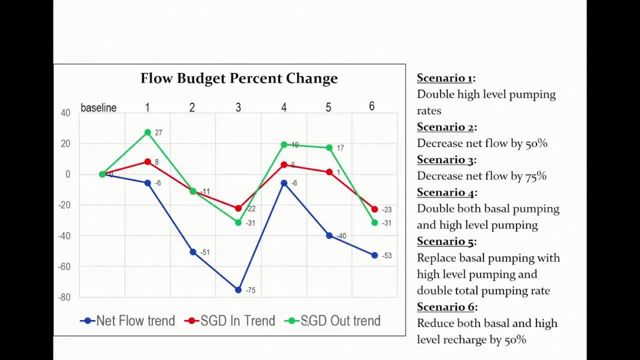 11%, etc. Then this is the green, Is the flow out Like here, increase 27% And, depending on your purpose, You can design Or accept the scenario. If you are interested in ecological factors, Then scenario one would be the best. 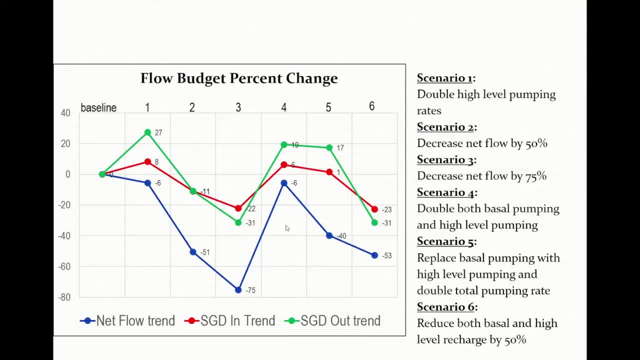 Give you increase In freshwater flow to the ocean, But in the meantime You have increase in inland Saltwater. So basically, Based on comparison To the baseline, You can choose whatever scenario Is appropriate for your needs. Then the final model. 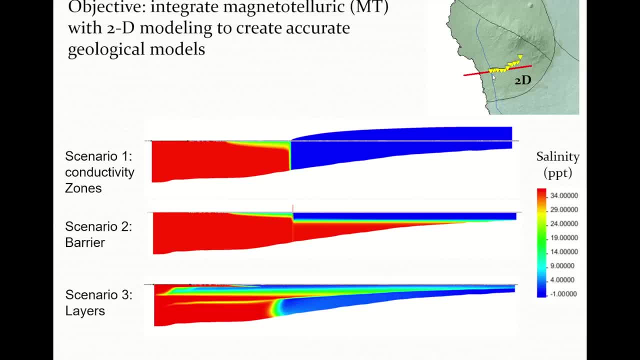 Has to do the cross section Across the site here And the objective Was to integrate Geophysical work With the 2D model, Try to build this Accurate geological model. So we had some scenarios Like different zones. 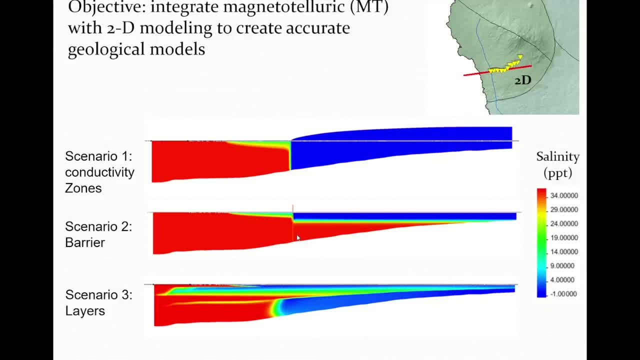 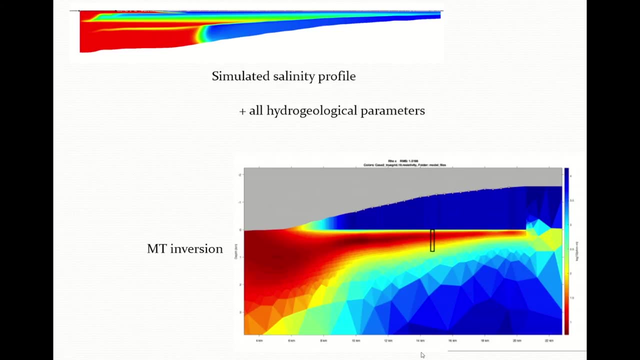 Different conductivity. Then here we have a vertical barrier, Then here we have layering Or different conductivity. So here is the salinity For the model. So we pass this to the Niels group, Which will invert it And estimate the MT. 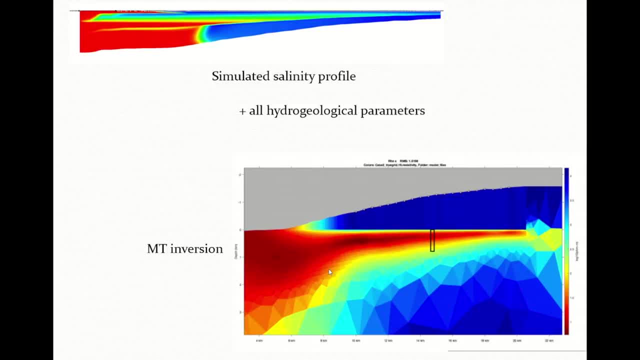 And using inversion To give you this profile here. So this is One of the examples And this is the respective MT measurements And we give them all the hydrological data Plus salinity And try to see Based on inversion. 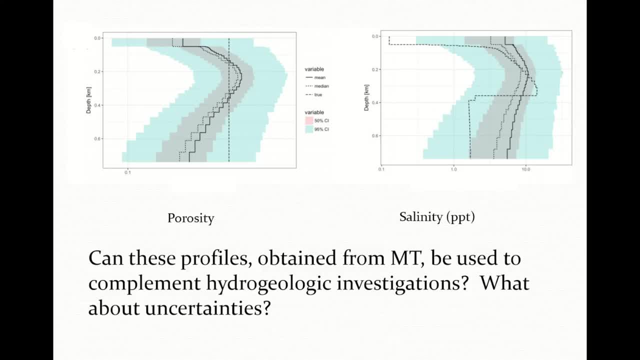 If we can invert it back To hydrological data. So, for example, Inverted MT, Then use MT to predict porosity And salinity And how accurate that inversion process is. So in other words, Can we use profiles Which obtained from MT inversion? 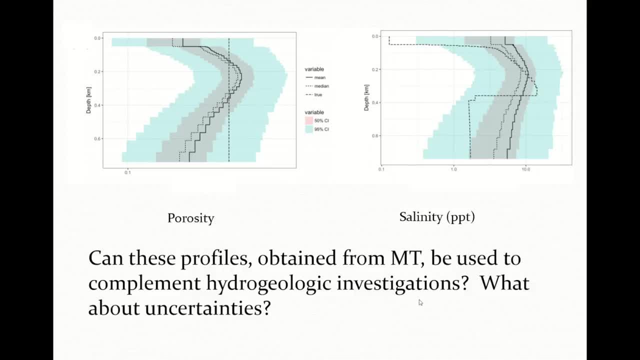 Can be used to complement Hydrological investigation And how the error Or uncertainty Can be affected by that. So here is the black Is the mean Of porosity Based on inversion, And here is the median And the through. 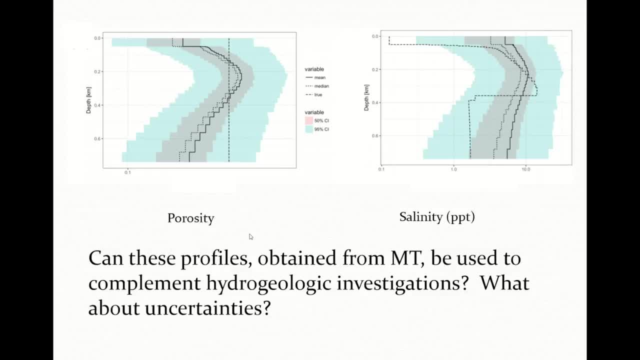 Which, basically, is This line here. So for salinity, This is the true, And the others are the same: Mean and median, And we can see The match is not great, But at least we have good idea When we can basically see. 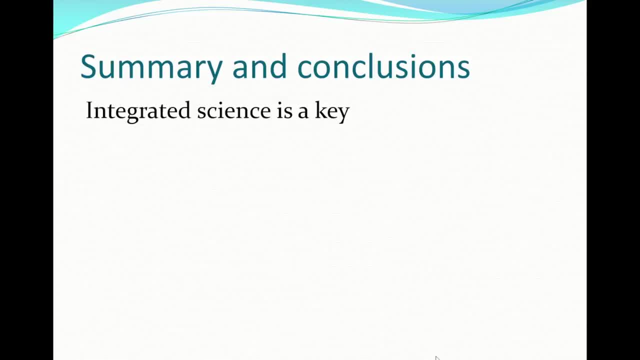 How we can improve on the technique As we go on. Okay, So integrated science is the key, Basically, due to the lack of information. We can integrate geophysical, Geochemical With numerical modeling For best assessment And reduction of uncertainties. 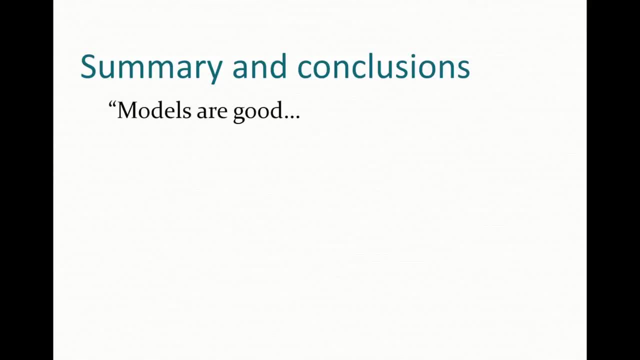 And I always tell my students: You aren't the ones to charge. The model can be great, But unless you are really careful, Things can go wrong. Okay, Thank you very much.